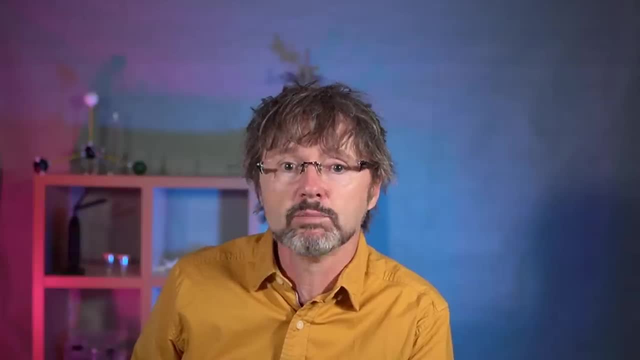 Now, if you're not already confident about atomic orbitals, you can combine these orbitals with each other to make the shapes and geometries we need to explain the shapes of molecules we see, and they are called hybridised orbitals. Importantly, these overlaps only occur between adjacent atoms. 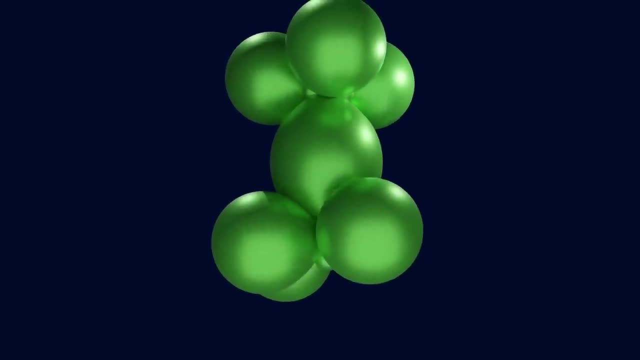 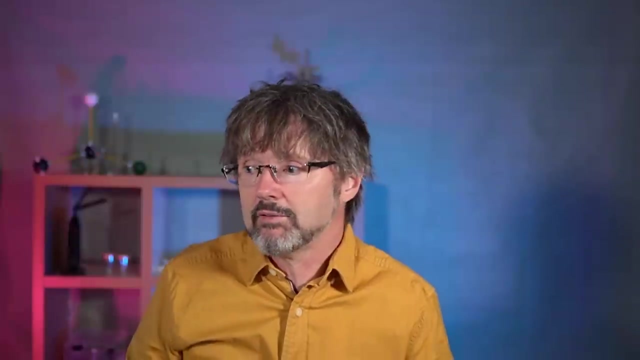 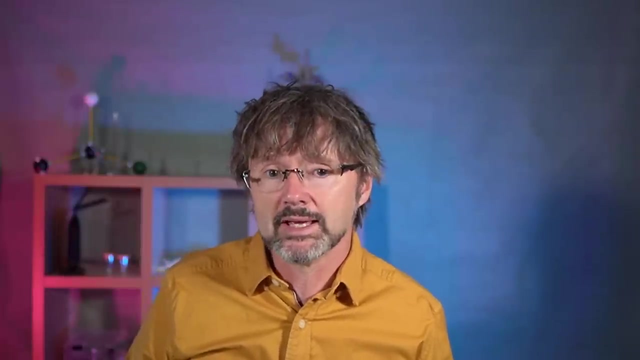 and we consider bonds to only occur between pairs of atoms at a time. That's great, but there are many things it doesn't explain. As a student, I could never understand, for example, why some atoms break the octet rule and others don't, And it's not very good for making predictions, for example with aromaticity. 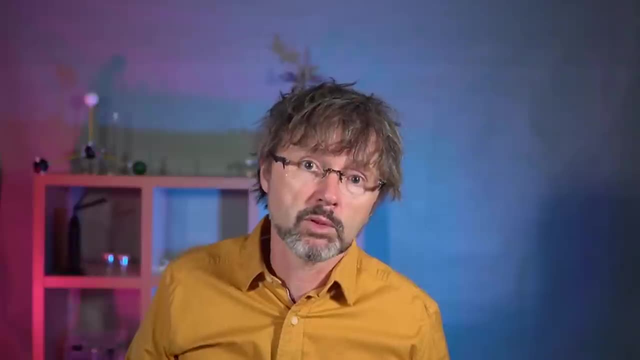 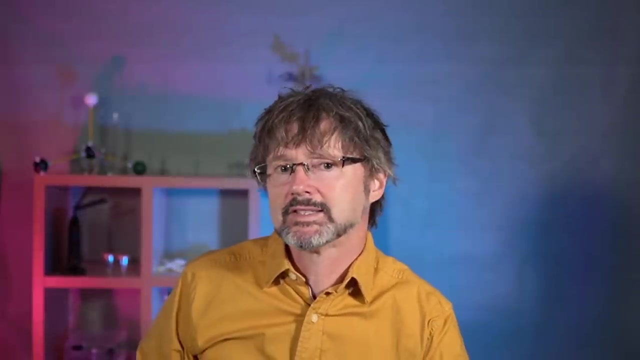 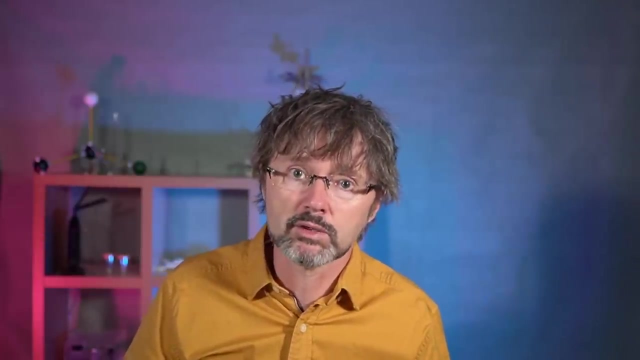 And sometimes it's just plain wrong. For example, the bonds are not the same. So what's a better explanation? Well, it's something called molecular orbital theory. This is a different explanation for how atoms make molecules. There certainly is some overlap with valence bond theory. but thinking of it as a different and complementary theory makes everything a lot easier to follow. So what is the big difference? In molecular orbital theory, there is a difference between atoms and molecules. In molecular orbital theory, there is a difference between atoms and molecules. 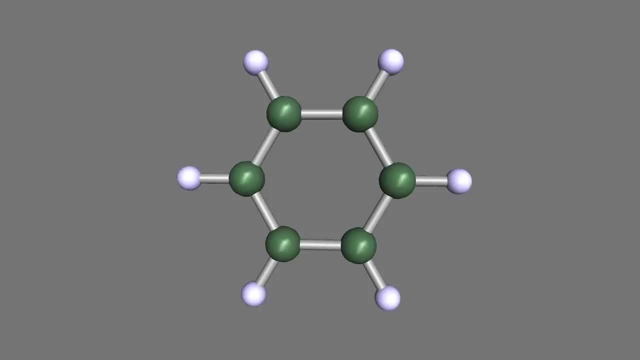 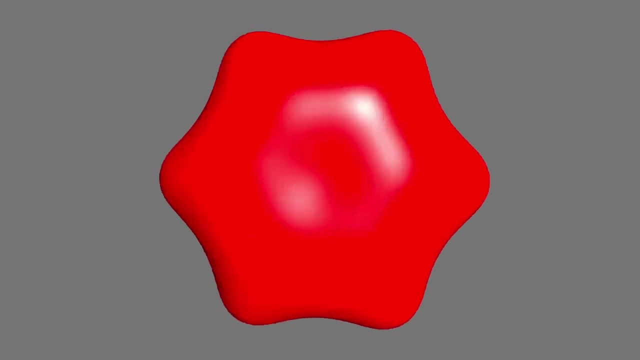 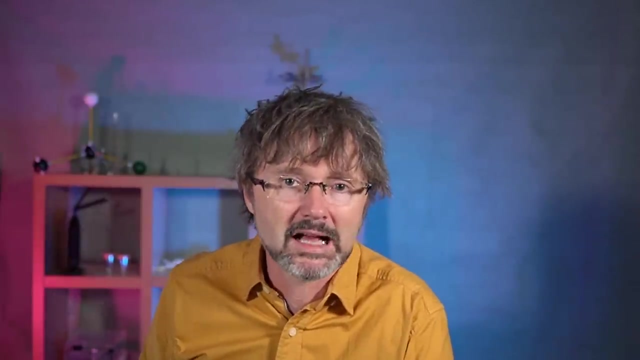 We imagine that all the atomic orbitals across all the atoms in the molecule overlap to make bigger orbitals that extend over the whole of the molecule. So let's take a look at how that works. And of course we are going to start with hydrogen gas because it's the simplest molecule. 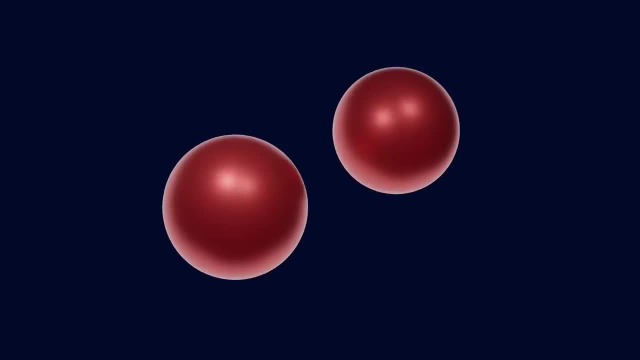 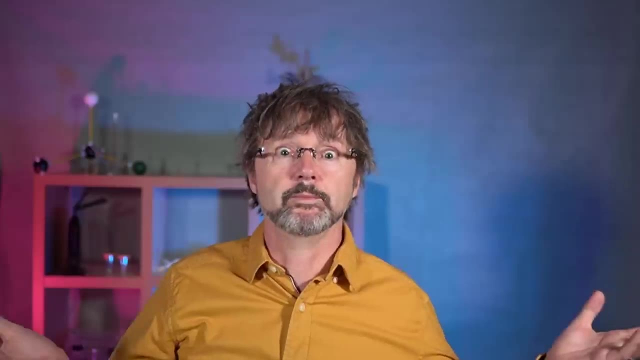 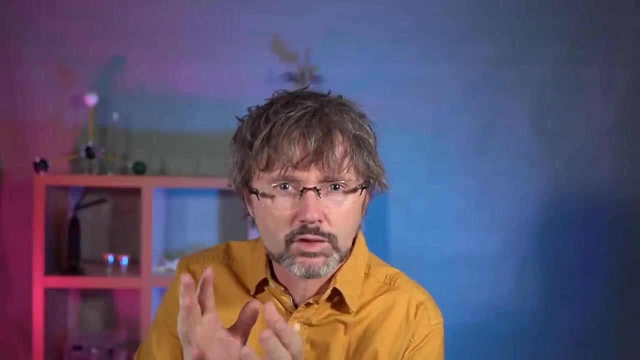 In H2,. the valence bond model is simple: The atoms overlap their 1s orbitals, share their electrons, forming a single bond. Whoopee Now. molecular orbital theory gives us a similar picture, but with slightly different consequences. 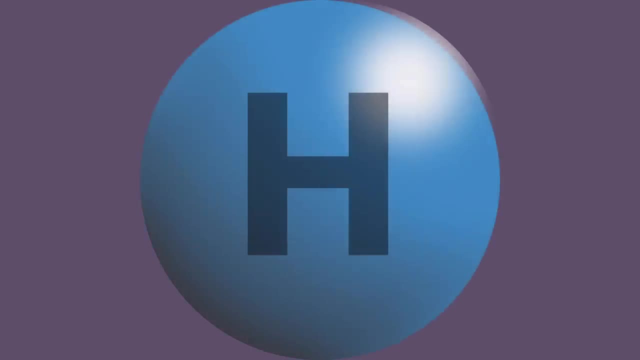 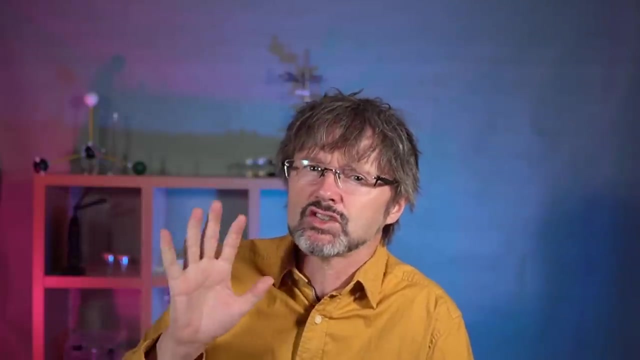 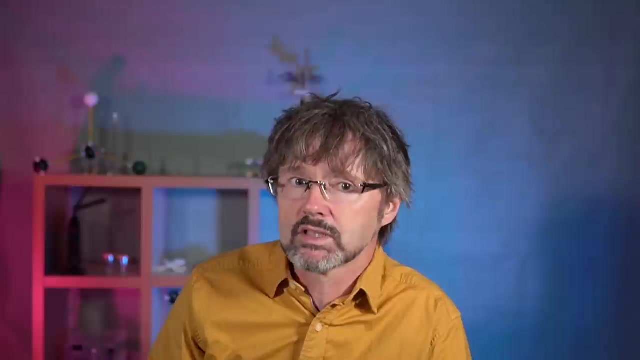 We can imagine that orbitals are three-dimensional oscillations, Oscillations of what? Well, probability, density, But let's just stick to calling it an oscillation for now. But where the orbital is oscillating the most is where we are most likely to find our electrons. 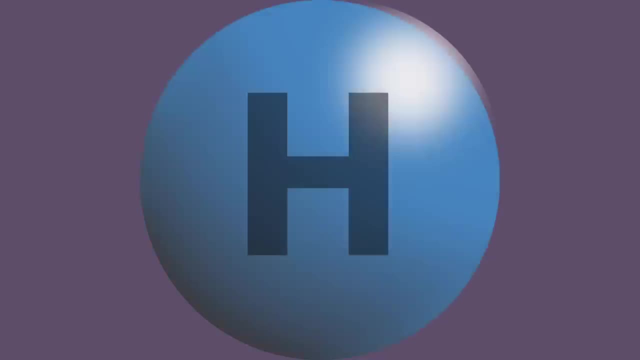 Now oscillations in quantum mechanics are called oscillations in quantum mechanics. Now oscillations in quantum mechanics are called oscillations in quantum mechanics. Now oscillations in quantum mechanics are called oscillations in quantum mechanics. Now, oscillations in quantum mechanics are nothing that we can visualize in our real world. 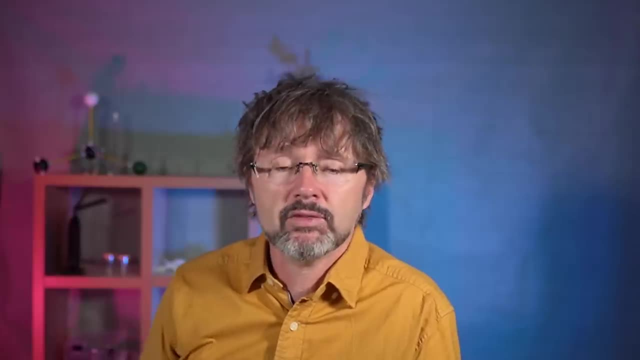 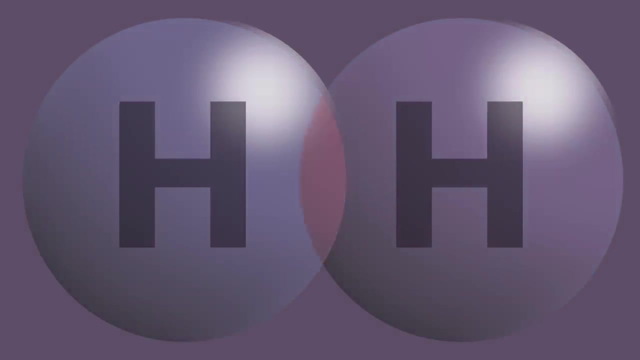 So I'm going to make some analogies In a simple wave phase just means: is it pointing up or is it pointing down? So now let's say that our two orbitals are either oscillating in phase and interfering constructively, or out of phase and interfering destructively. 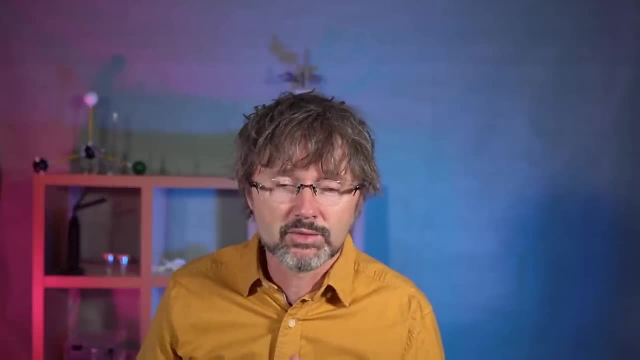 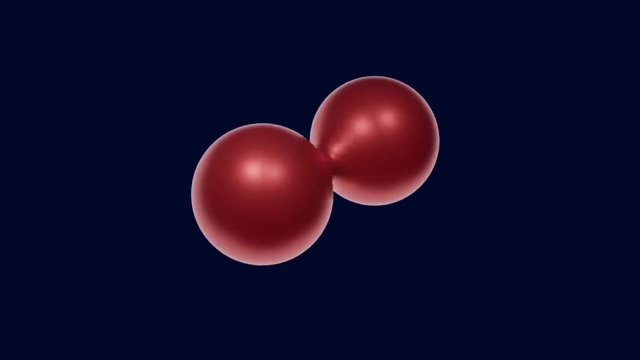 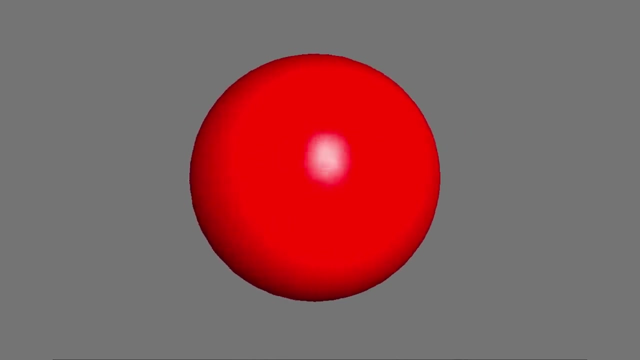 Anything in between is not a standing wave. So this gives us two possibilities for making our combined molecular orbitals. When they're in phase, the resulting molecular orbital extends over the whole of the molecule. We call this orbital a bonding orbital because it holds the atoms together. 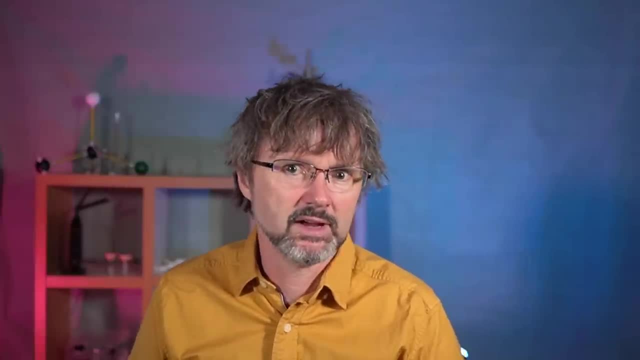 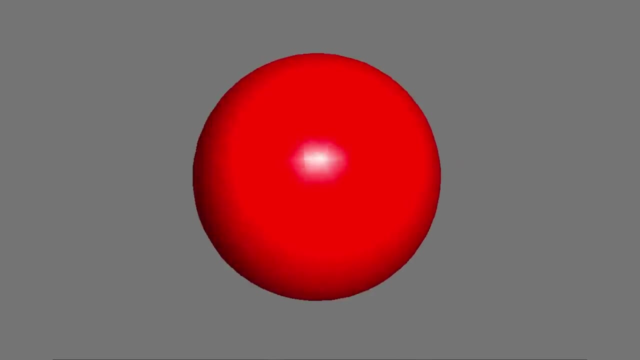 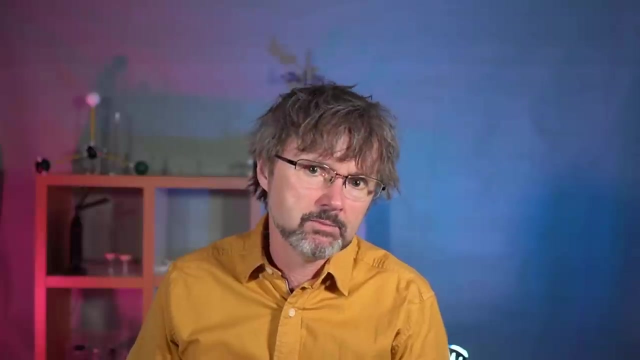 Now, remember, an orbital is not a container of any kind, A cloud is a better way to imagine it- And this hard surface just represents a certain value of probability of finding an electron. So if I want to change that probability, I can just move the slider to the left or to the right. 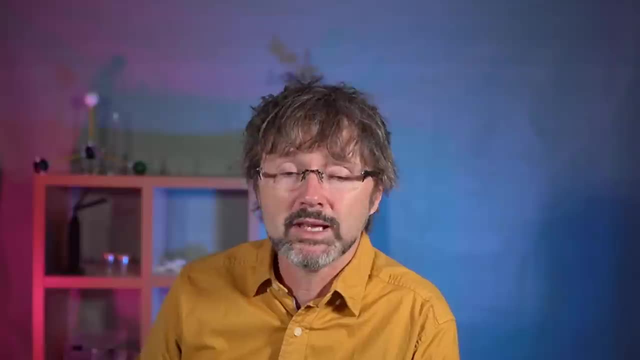 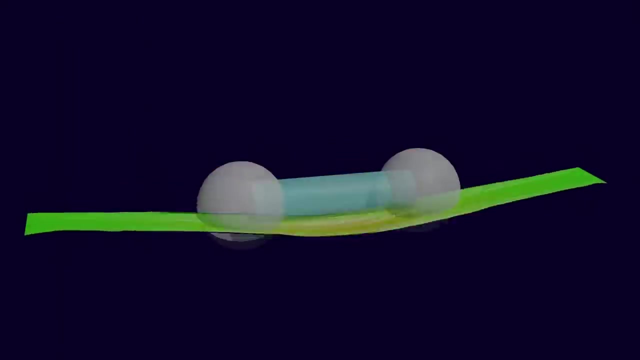 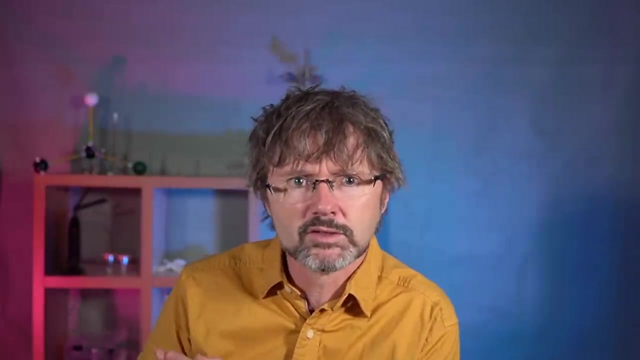 and it just makes the shell grow bigger or smaller. And we can make an analogy of that bonding orbital with this oscillating band. Where the band oscillates the most is where we find the greatest electron density. Okay, so that's not so different to our normal valence bond theory. so far, 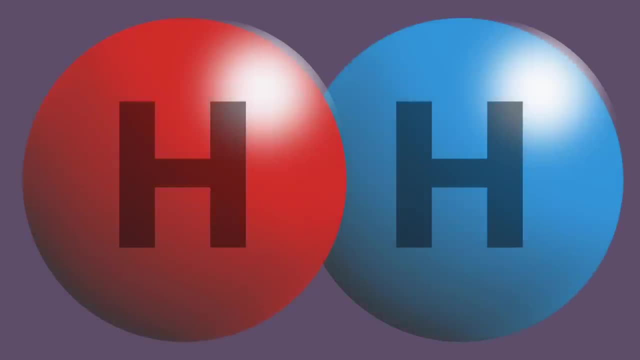 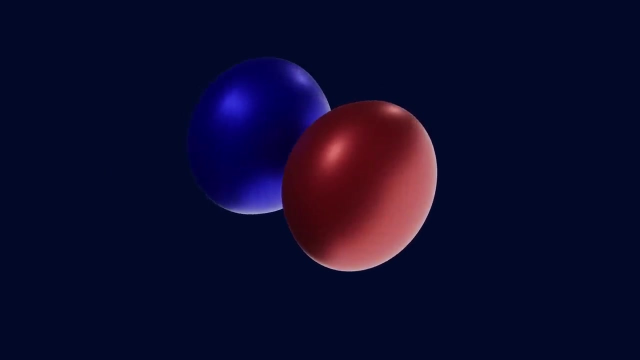 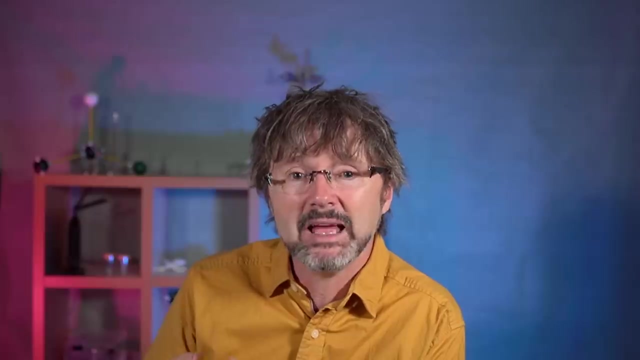 But now look what happens when the two atomic orbitals have opposite phases. Now they cancel each other out Where they overlap And we end up with more electron density outside the two nuclei. What this does is pull the nuclei apart and it makes an anti-bonding orbital that breaks up the molecule. 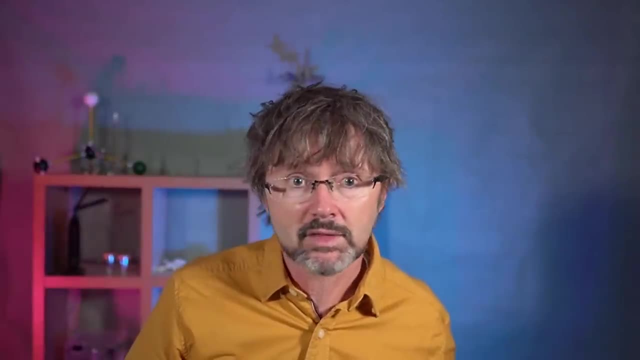 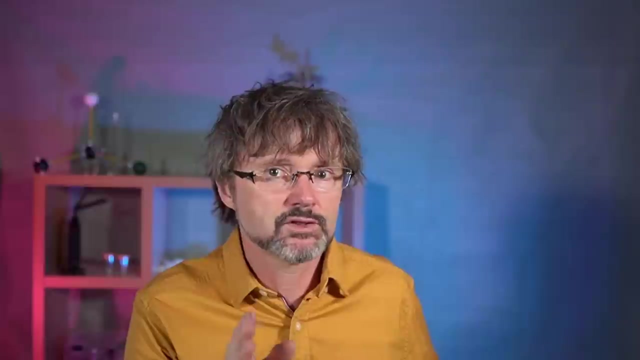 It's literally the opposite of a chemical bond. That's something that we absolutely don't have in valence bond theory. Now it looks like we have two orbitals, but we don't. They are two lobes of the same orbital. 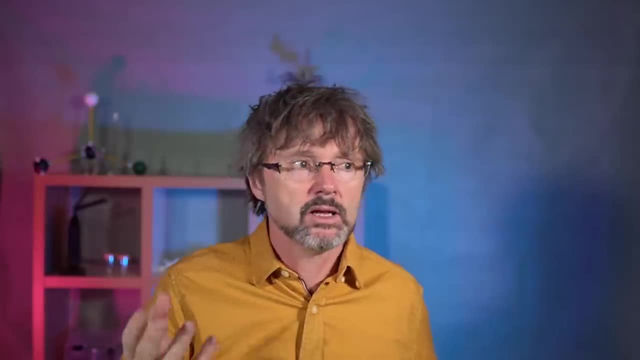 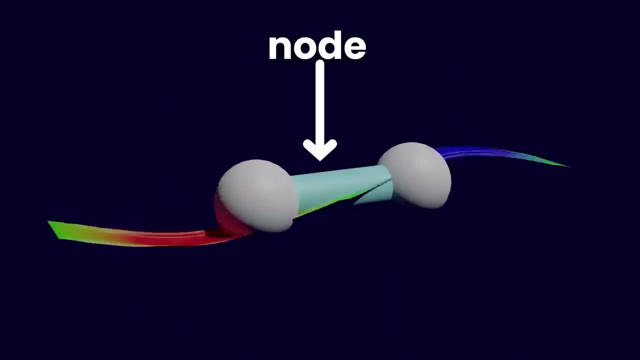 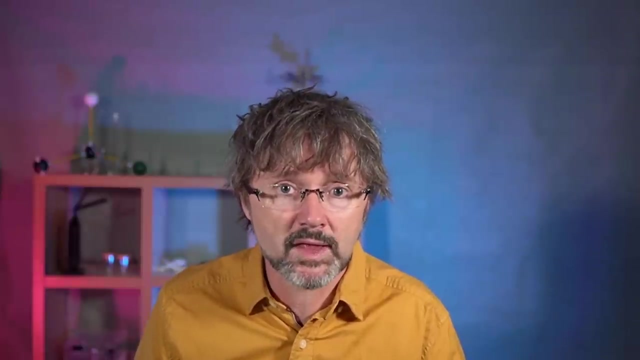 but they have different phases, A bit like the p orbitals on atoms. We can visualize it as being similar to this ribbon vibrating with a node in the center. And secondly, because it's one orbital, there is only space for two electrons there. 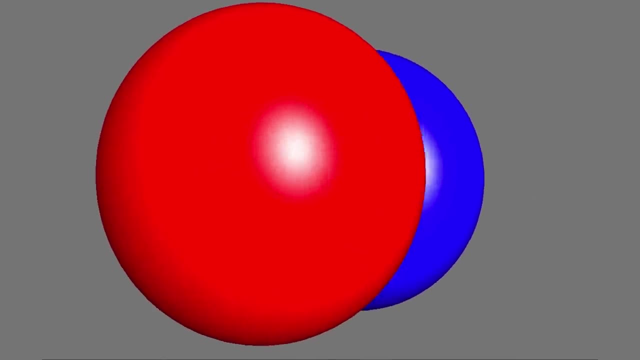 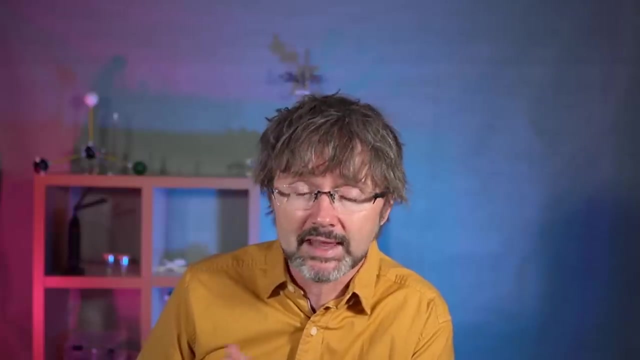 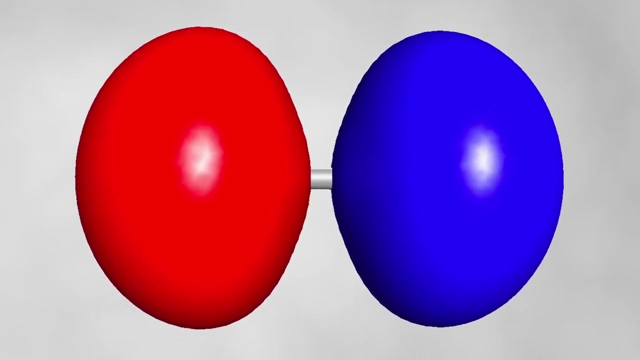 And thirdly, remember that although this picture shows a solid shape, the orbital is better thought of as a cloud. We can find electrons crossing the gap in the middle, but we're much more likely to find them somewhere inside the solid shape. So let's take a closer look and see how it all works. 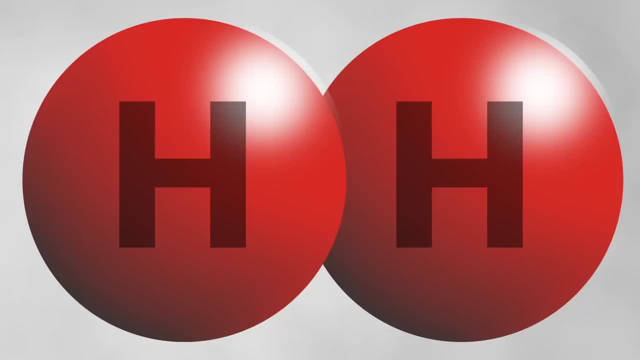 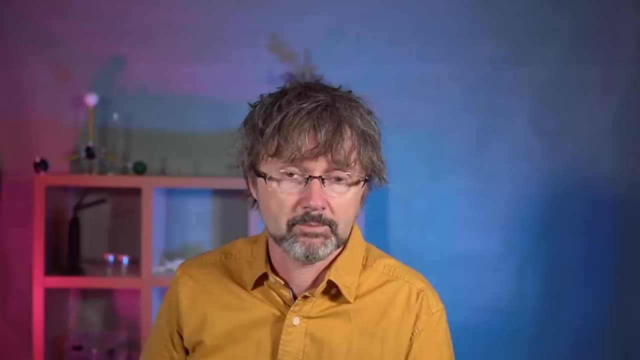 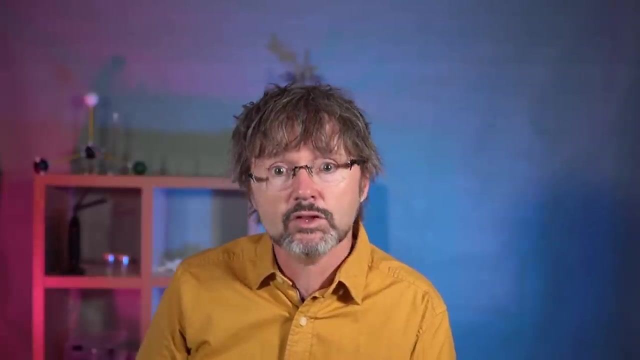 Firstly, we started with two atomic orbitals and they overlap to give us two molecular orbitals. That's a fundamental rule in molecular orbital theory: However many atomic orbitals we start with is the number of molecular orbitals. we finish with Knowing that at the start. we have two or three electrons in the same atom. it makes everything so much simpler later. It also removes one of the big problems with valence bond theory, expanded octets and expanded eighteen electrontets. With molecular orbital theory we don't need to find ways to explain how certain atoms get too many electrons. 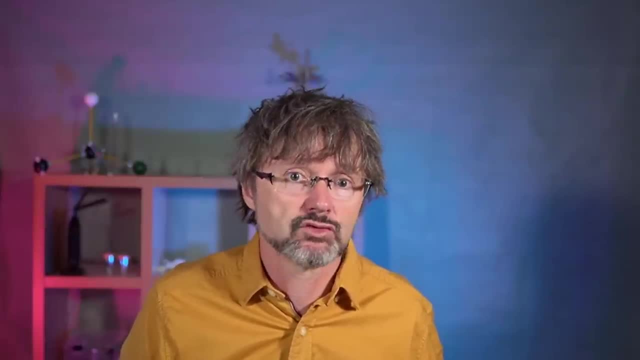 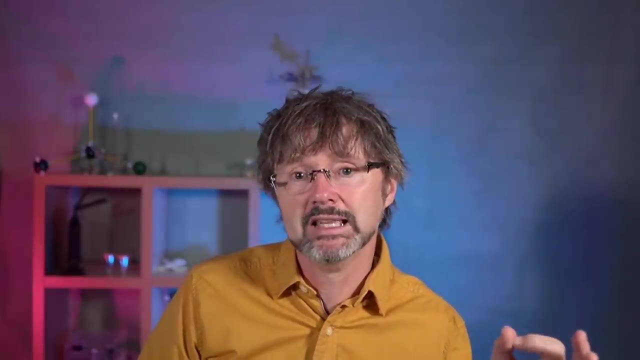 Instead, we can see that all of the atoms which are in the same orbital structure have the same amount of potential energy for the electrons that they have Next up. a crucial aspect of orbitals is how much potential energy electrons have when they occupy them. 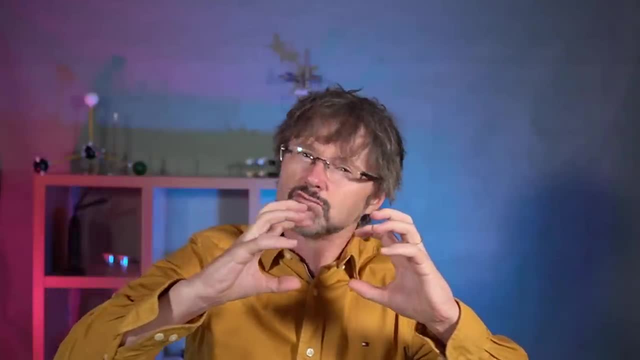 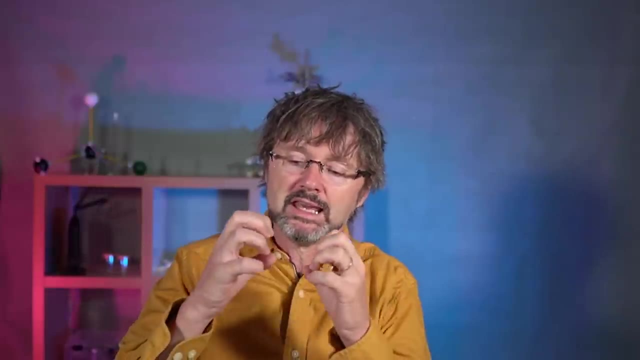 Potential energy comes from pulling apart things that are attracted to each other, or by pushing together things that repel each other. So our electrons will have less potential energy the closer they get to positive charges. Since the two electrons sitting in the bonding orbital 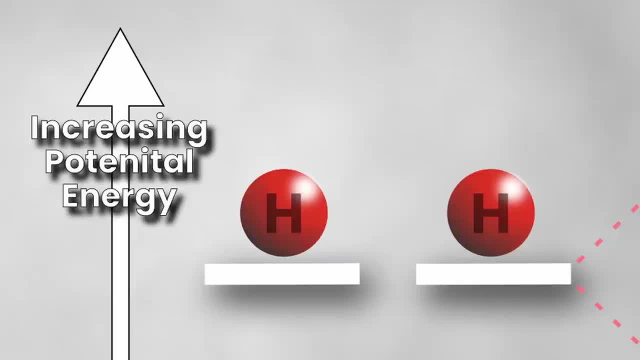 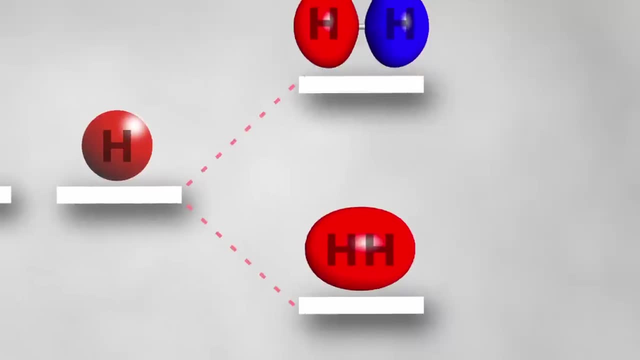 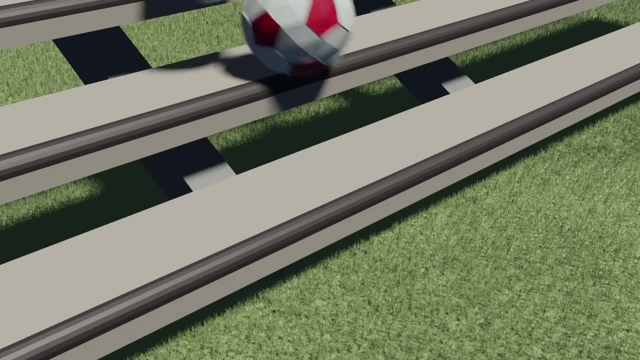 are close to two nuclei at the same time, they will have less potential energy than electrons sitting in the anti-bonding orbital, where they're only close to one nucleus at a time and further away from it anyway. Now remember that systems with less potential energy are more stable. because they have less energy to do things like break apart. That's one half of what stability is. Furthermore, the anti-bonding orbital will have less potential energy than electrons sitting in the anti-bonding orbital. The anti-bonding orbital has a node in the middle. 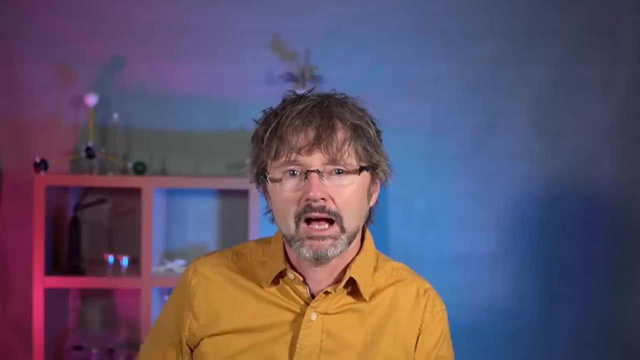 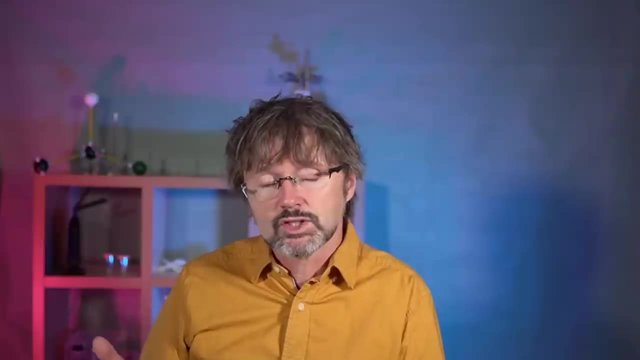 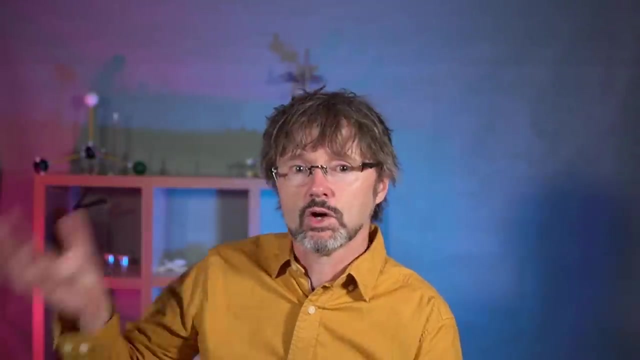 a space with little to no electron density. Having more nodes for a given size is often associated with higher potential energies. For now we'll just say that those nodes give orbitals a shape that keeps electrons further from the nucleus. So we put all this together. 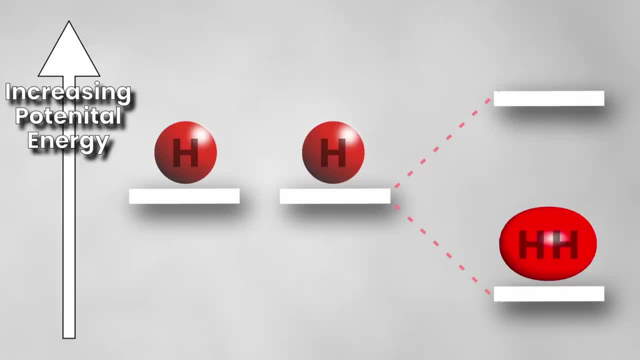 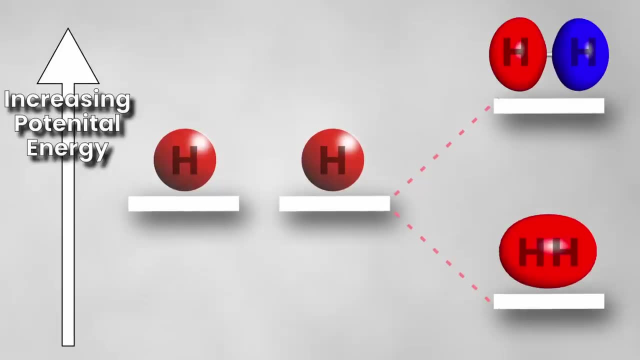 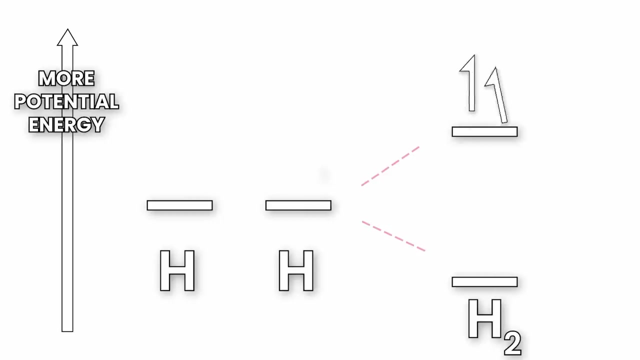 and see that bonding orbitals have electrons with less potential energy than when they are in separate nodes And much less than when they are in the anti-bonding orbital. And remember that electrons will always drop into the lowest energy orbital that they can. 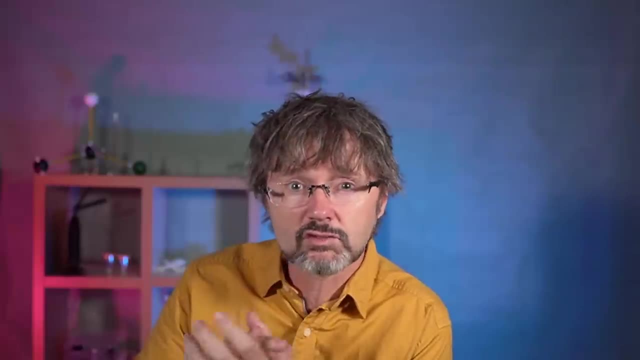 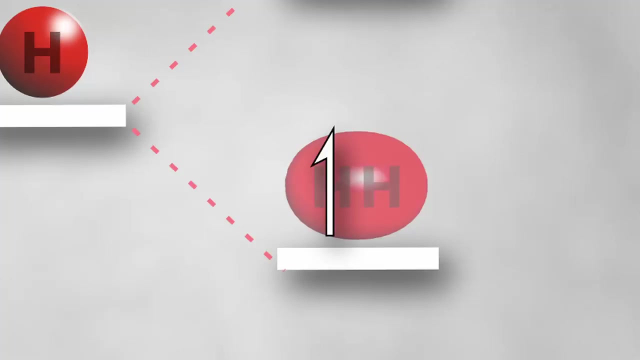 But if some UV light of just the right wavelength hits the molecule, it can excite one of the electrons to the anti-bonding orbital. The low energy electron gluing the nuclei together is now cancelled out by the high energy electron pulling them apart. 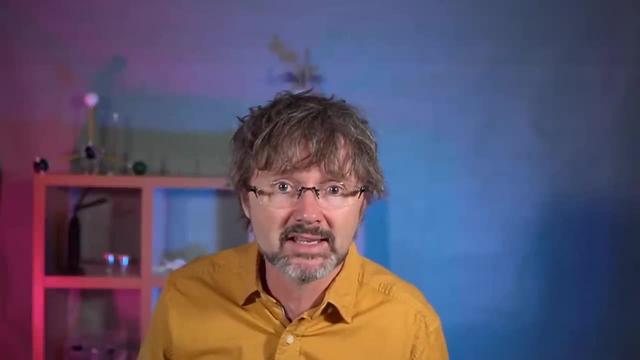 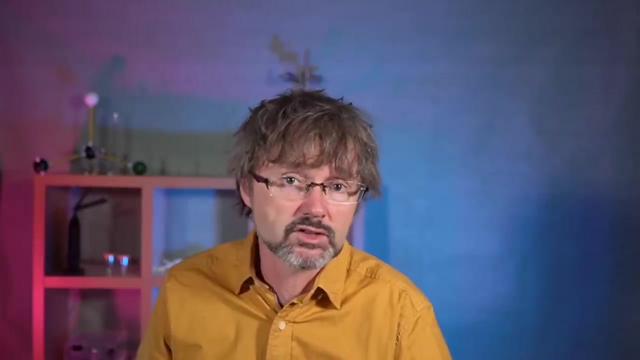 And there is no longer any benefit to the atoms staying together. So the atoms will fly apart because of entropy- which is a fancy-pantsy way of saying that they will just go everywhere that they can go- And ultraviolet-like, breaking up chemical bonds. 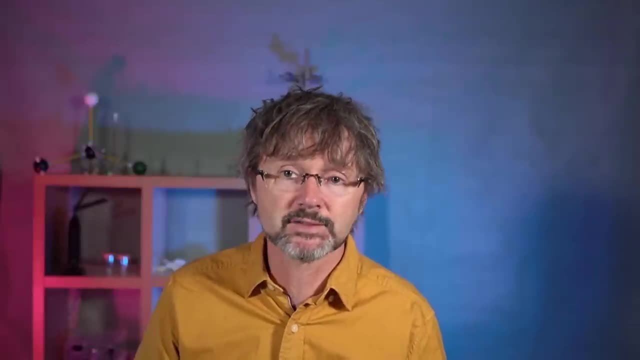 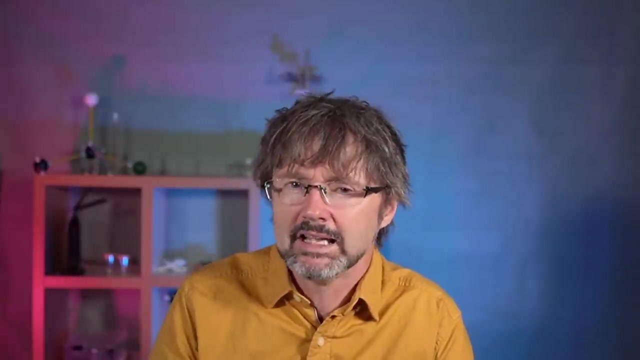 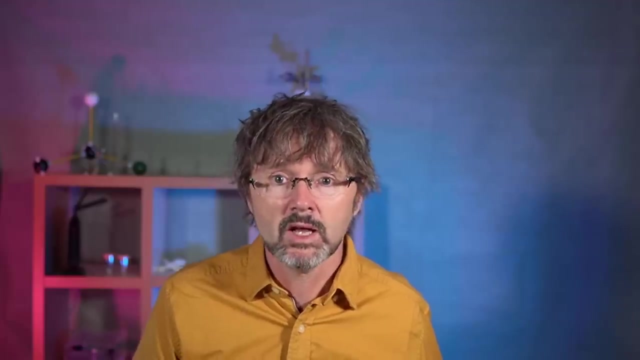 is exactly why it's so dangerous to bags of chemicals like us. But how does all this work with helium, our other first row element? In valence bond theory? we simply say that helium has a full principal quantum shell, so it doesn't do chemistry. 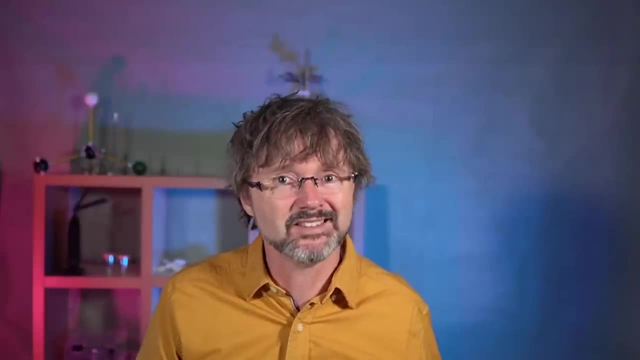 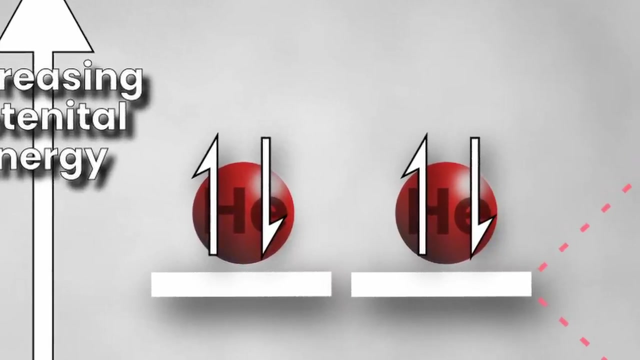 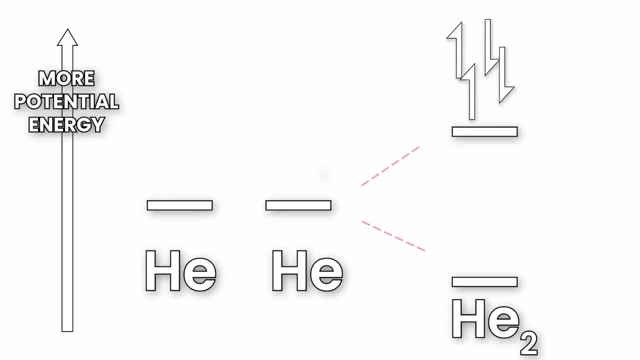 But molecular orbital theory explains this in a different way. We have the same atomic orbitals as hydrogen, but now we have four electrons to fill our two molecular orbitals. That means two drop into the bonding orbital that pulls the nuclei together, but two are left in the anti-bonding orbital that pulls them apart. 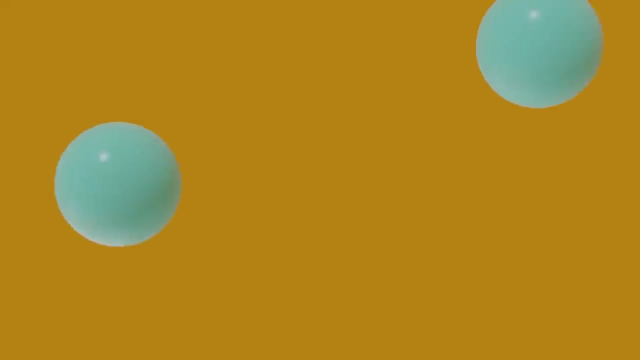 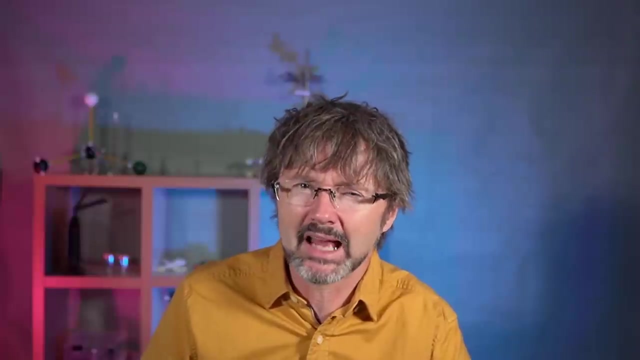 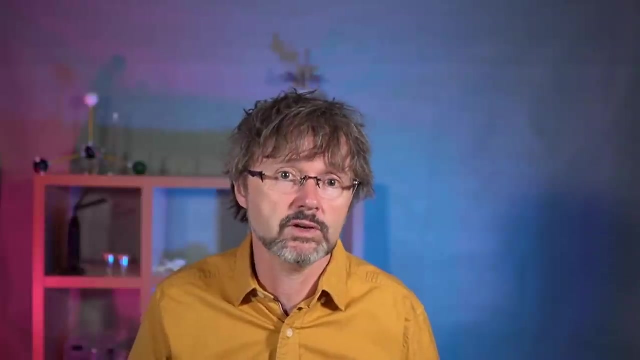 So now there is no incentive for the atoms to stay together and they'll simply fly apart. Now we say that helium doesn't do any chemistry. but actually it does. And not only that, it did the first chemistry ever in the history of the universe. If we overlap a helium atom with a positive hydrogen ion, a proton, we only have two electrons. There isn't much benefit for the electrons spreading themselves over two nuclei instead of one, so it falls apart then. But we have detected this molecule in space. 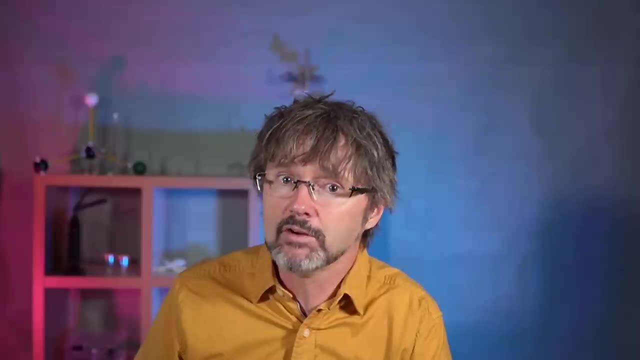 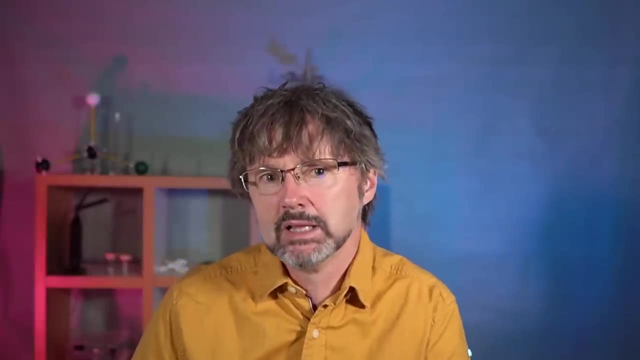 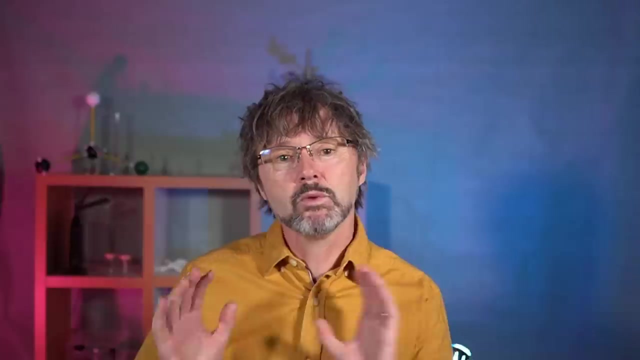 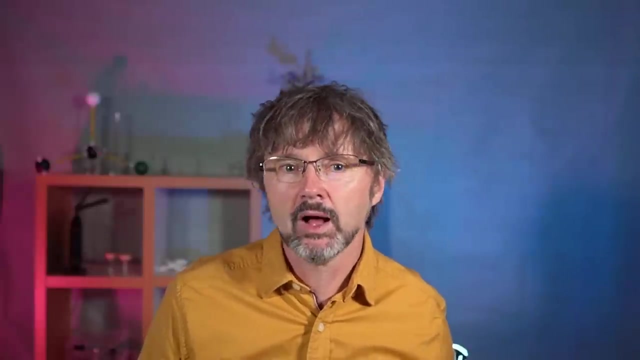 and it's very likely to have been the first ever molecule, even before H2.. So that's the basics, But what is it that makes molecular orbital theory so special? Well, let's start by looking at dioxygen O2.. Now, I'm not going to go into details of which atomic orbitals make which molecular orbitals. 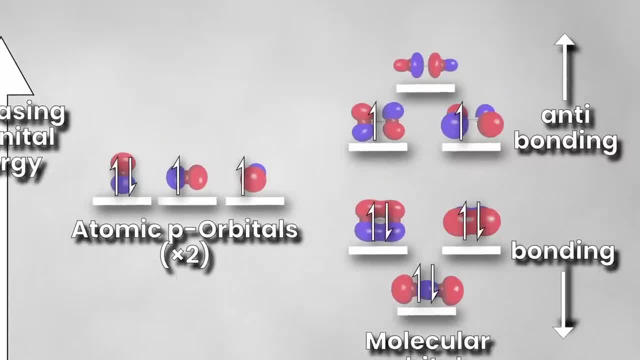 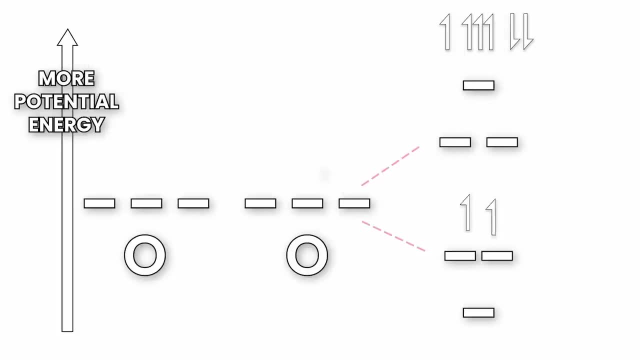 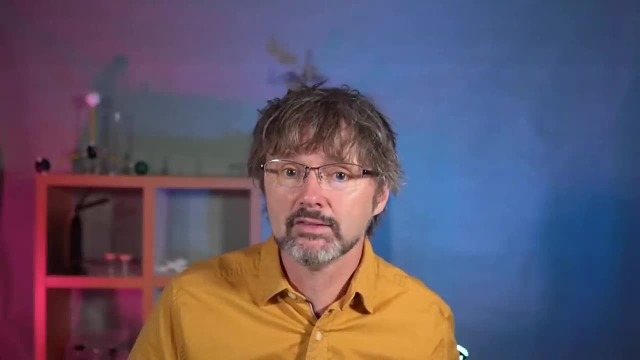 I just want to draw your attention to the top of our little energy diagram here. As we drop electrons into the molecular orbitals, we still have two electrons left over after filling up all the bonding orbitals, But the next orbitals are anti-bonding orbitals that both have the same energy. 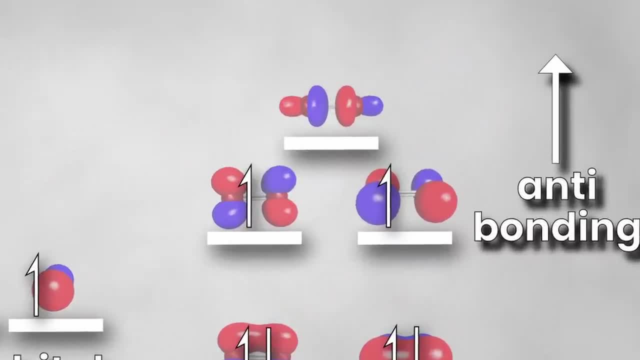 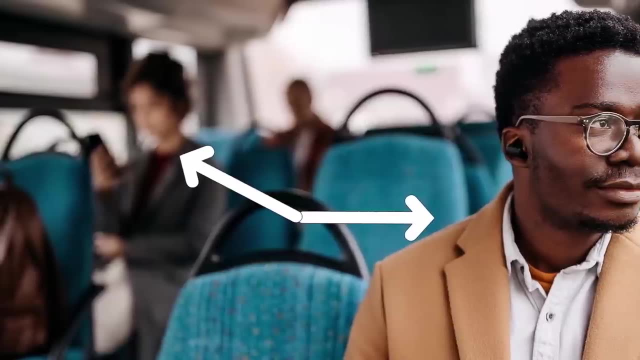 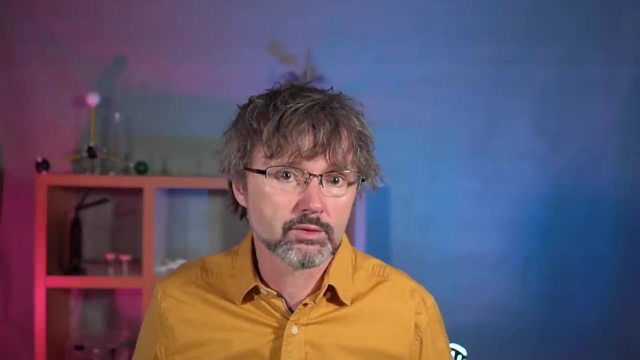 So those electrons won't sit together in the same orbital. they'll sit in the two orbitals separately, Just like when you're on a bus: you won't sit next to a stranger if there's an empty seat just across the aisle. And that means that, according to molecular orbital theory, 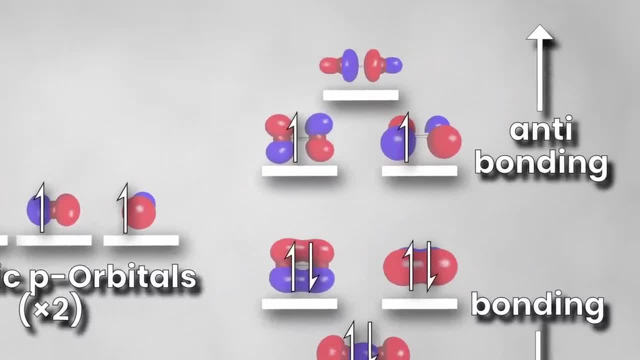 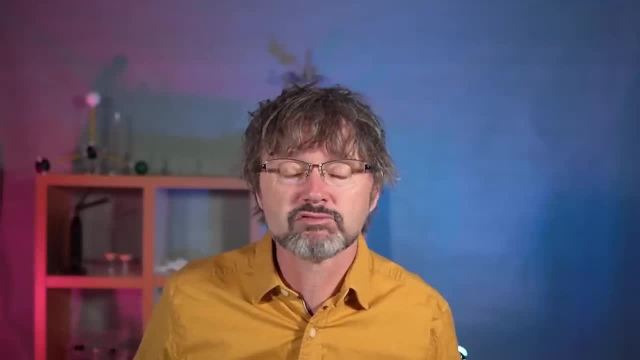 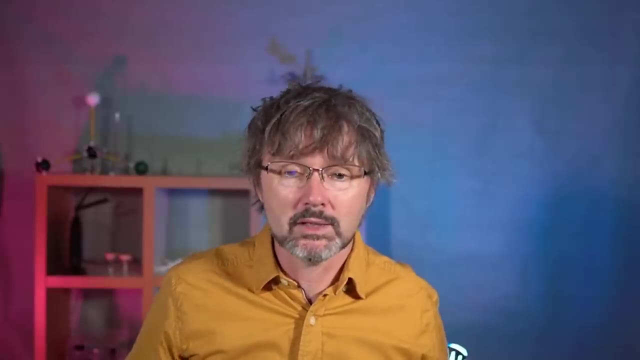 oxygen gas has two unpaired electrons. In other words, it's a double radical, Which is completely different to valence bond theory, which predicts a double bond with two lone pairs on either oxygen atom. So which one's right? Well, it's molecular orbital theory. 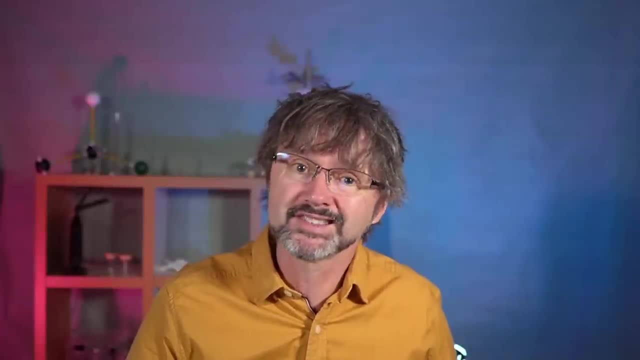 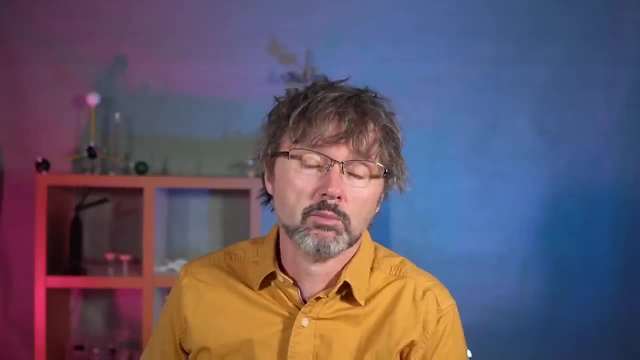 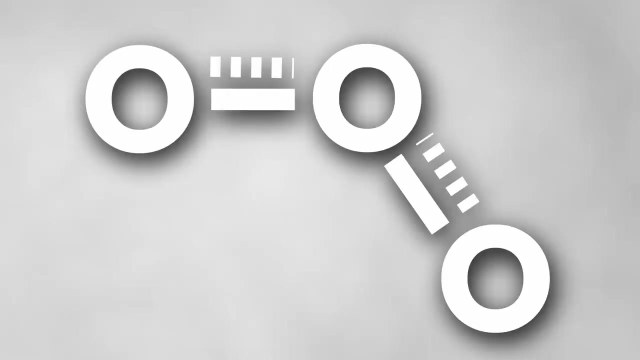 We can tell, because the unpaired electrons don't just give oxygen a faint blue colour, they also make it slightly magnetic. Now, diatomic molecules are fairly simple, So let's extend our oxygen molecule by one atom to make ozone, And after that we'll have a look at some really kooky examples. 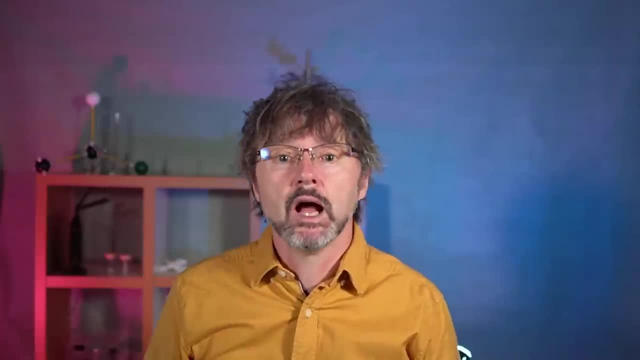 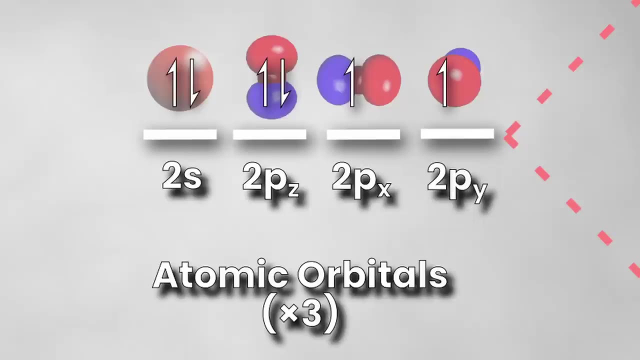 But before I forget, if you click on the like button, it'll help me make more videos, Thank you. Now, in ozone, our s orbitals and our p orbitals link up to make molecular orbitals that run up and down the whole molecule. 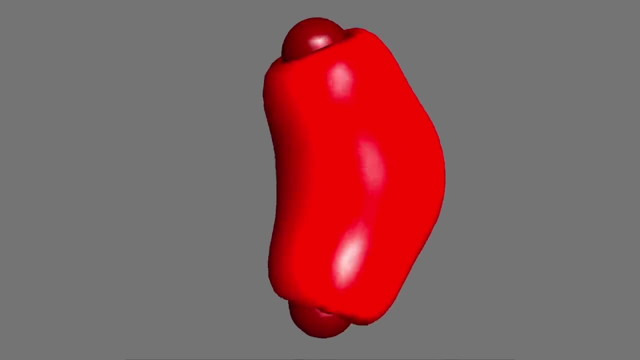 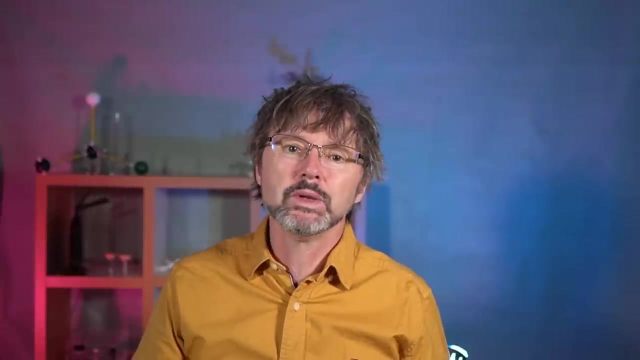 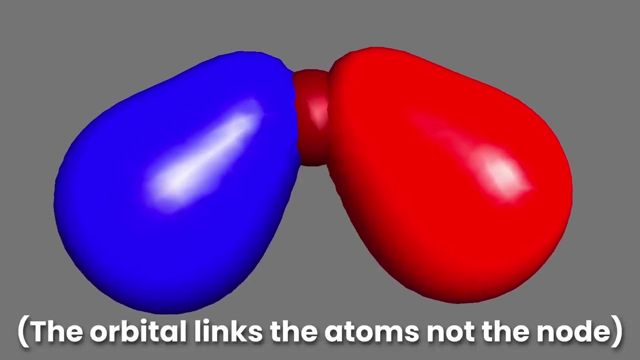 For example, we can get this lovely tube shaped bonding orbital. Now, as we make the different combinations of atomic orbitals, we get nodes of low electron density like this one that links both the outside atoms directly to the central atom, but with a space. 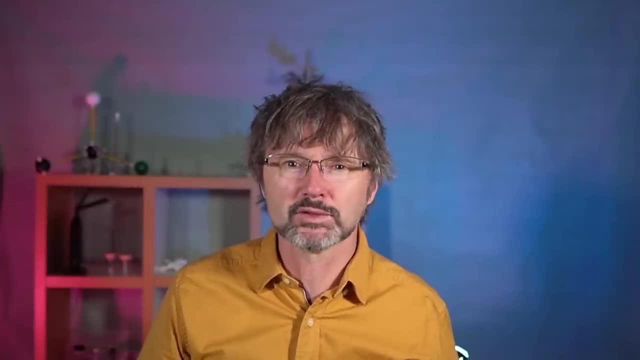 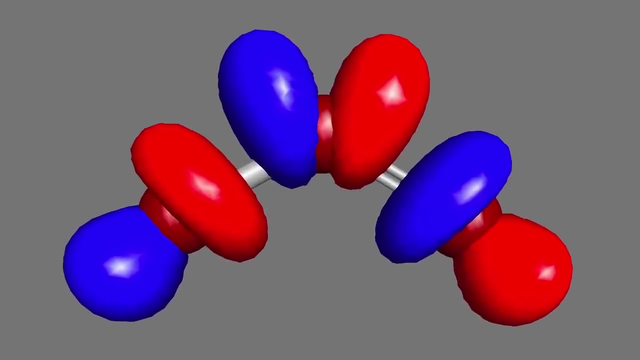 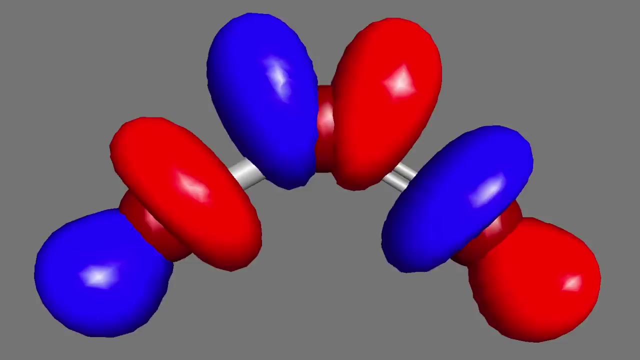 right in the middle. But it's the antibonding orbitals that really show us the fun of molecular orbital theory. This is the antibonding orbital version of the tubular bonding orbital. Notice how it has nodes all over the place, but particularly between the atoms. 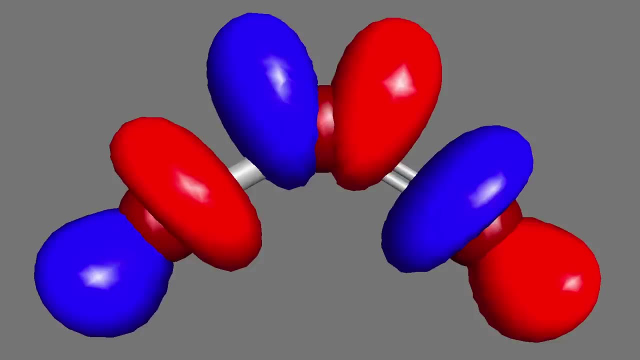 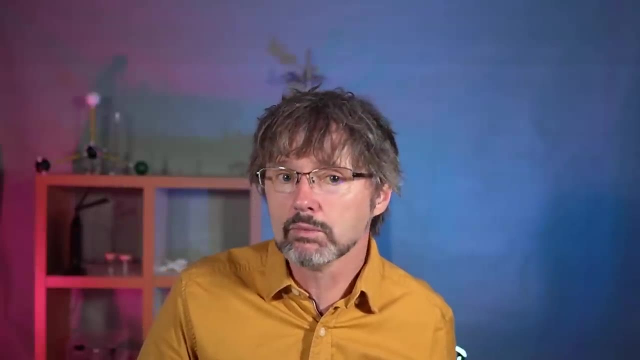 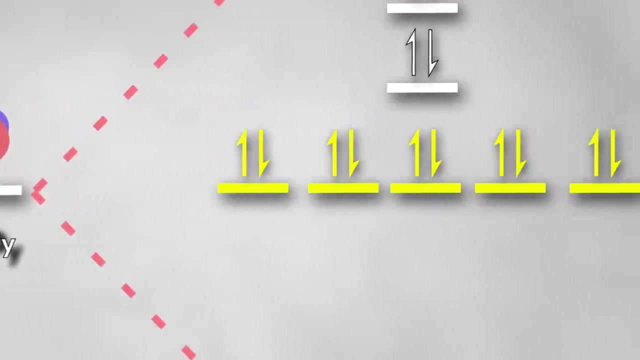 meaning there is empty space with virtually no electron density between the atoms now. But now we've got more than two atoms. We can also see non-node. These are molecular orbitals that aren't very different in energy compared to the separate atomic orbitals. 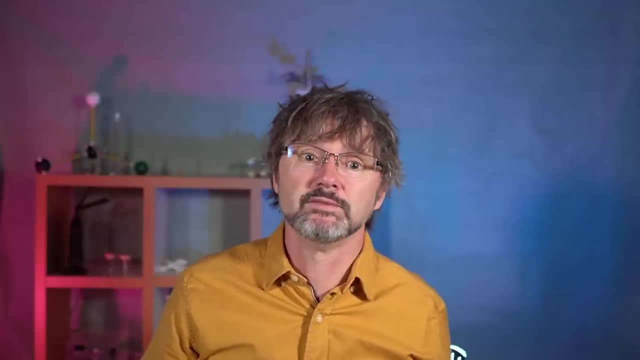 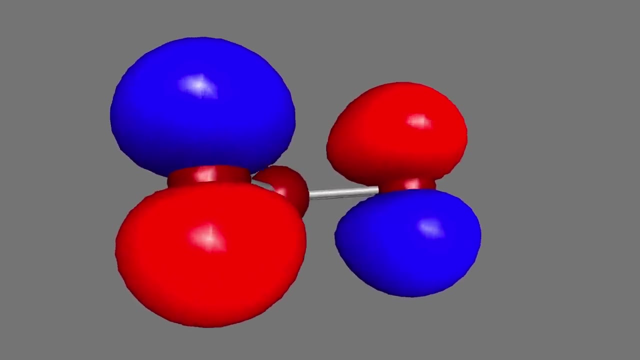 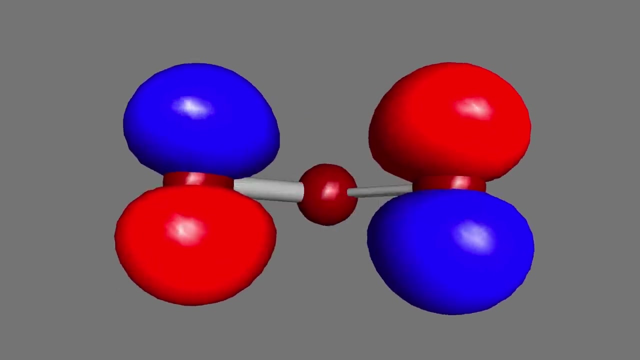 And that's because the constructive and destructive interference basically cancel each other out. We can see from this orbital, for example, that electron density sitting directly above and below the atoms doesn't really do anything to pull them together or apart. And I'm going to repeat this. 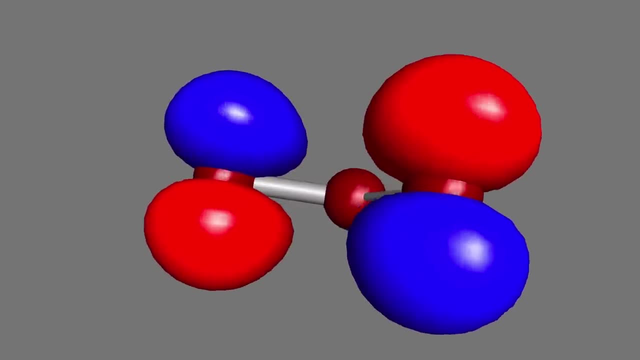 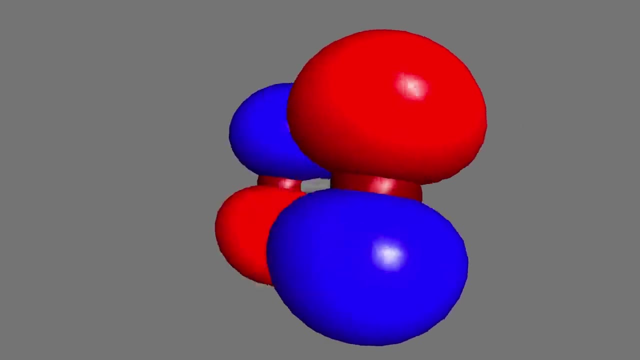 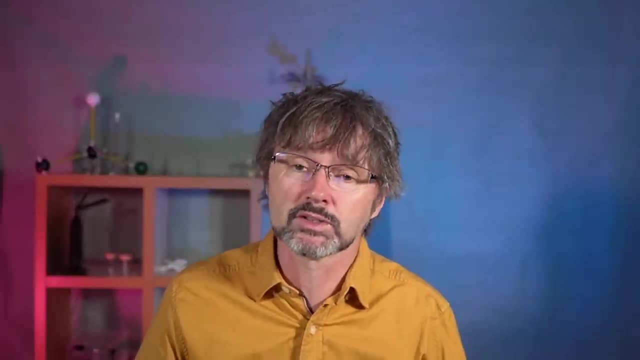 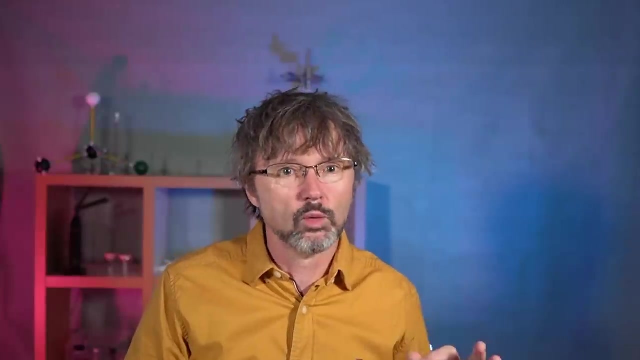 And if you're interested in the details of how atomic orbitals combine to make these molecular orbitals, I've put a link in the description. So now we've seen how molecular orbitals extend over a whole molecule. Let's have some fun. 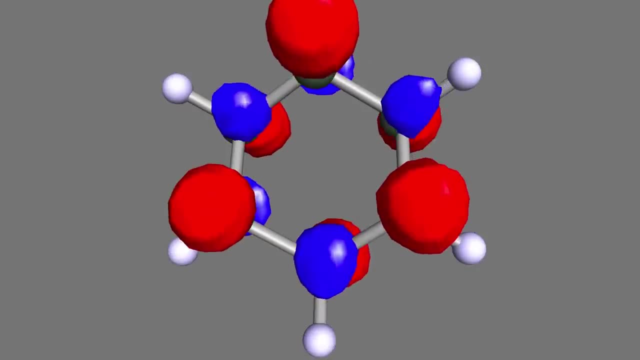 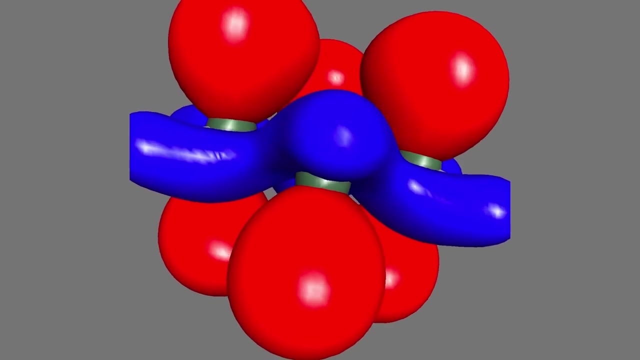 Can you spot what molecule it is? It is, of course, cyclohexane. Once again, this is one single orbital with only two electrons in it. So now, how about this molecule? Can you guess what it is before I show you? 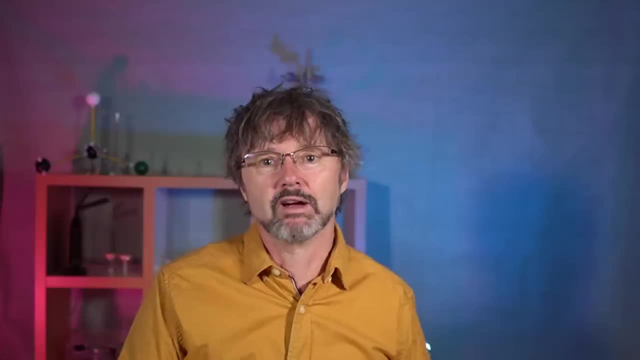 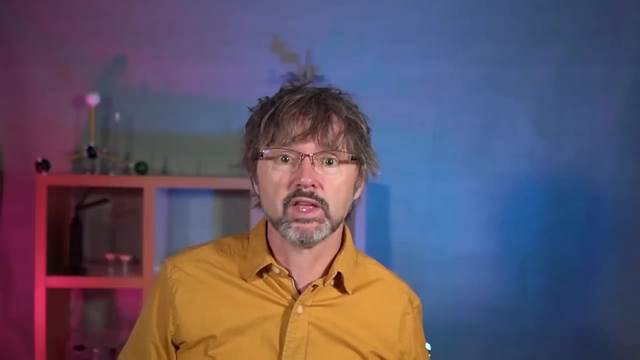 That's right, It's benzene. Now, benzene is directly related to cyclohexane. It's just lost six of the hydrogens. And sure, in valence bond theory that means it should be like hexane, But with some double bonds. 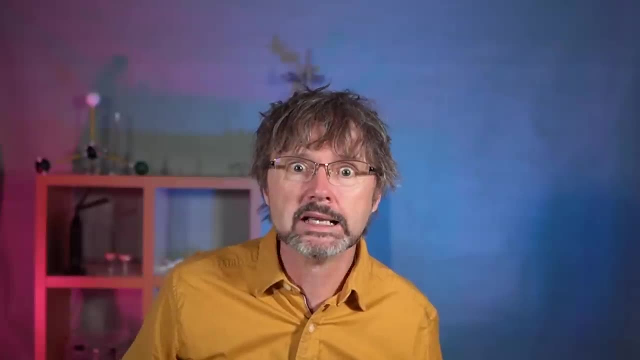 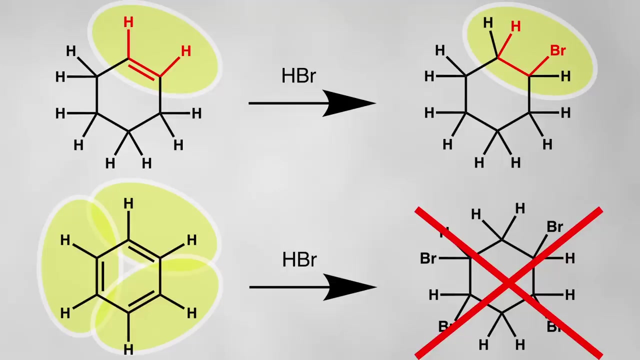 But it's not a bit different, It's completely different. It's far more stable than it should be. It doesn't do double bond chemistry And all the bonds are the same length, instead of having different lengths for single and double bonds. 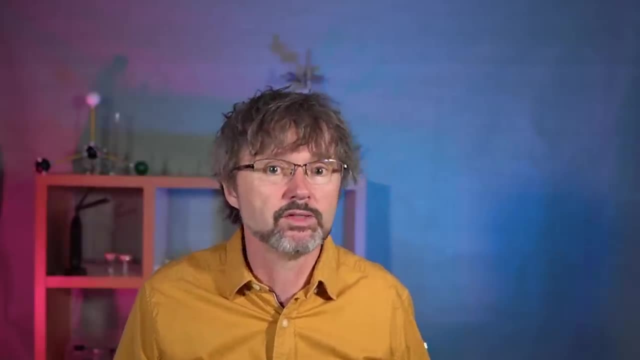 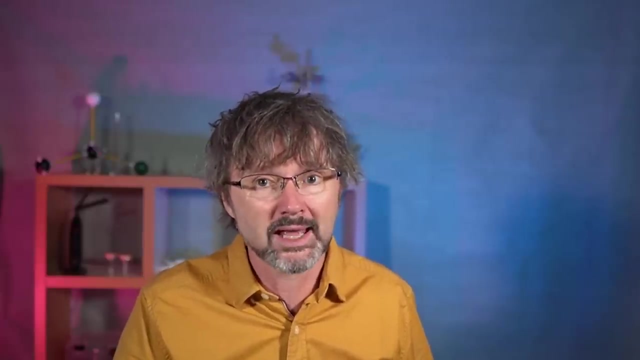 Not to mention the weird stuff it does when we analyse it with spectroscopy. This is a phenomenon called aromaticity, And it's actually much more complicated than the textbooks tell us. So let me know in the comments if you want a dedicated video. 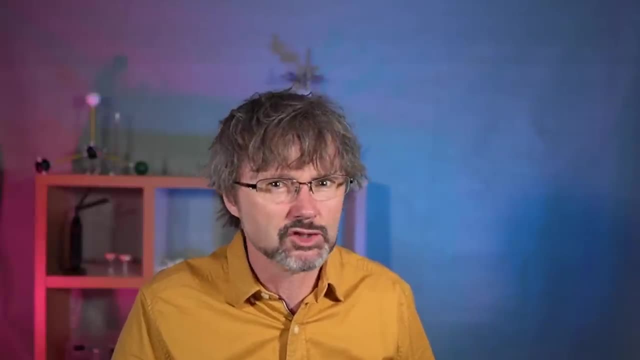 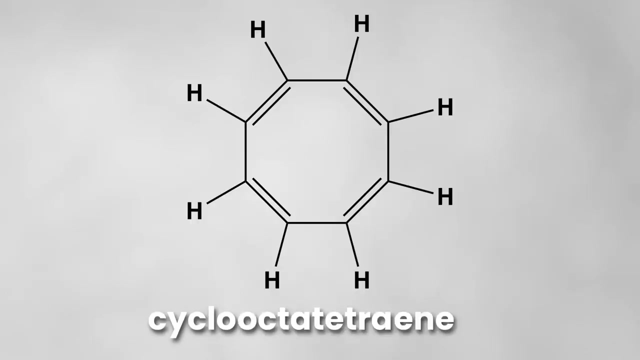 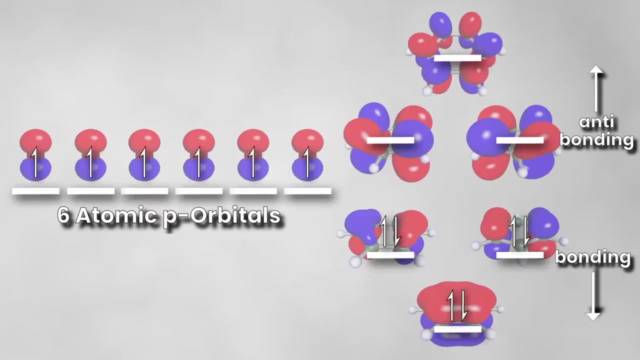 But for now valence bond theory doesn't do a great job of explaining why benzene is aromatic while cyclooctatetraene isn't. But in molecular orbital theory we can see that benzene and other aromatic molecules have all their electrons in bonding orbitals. 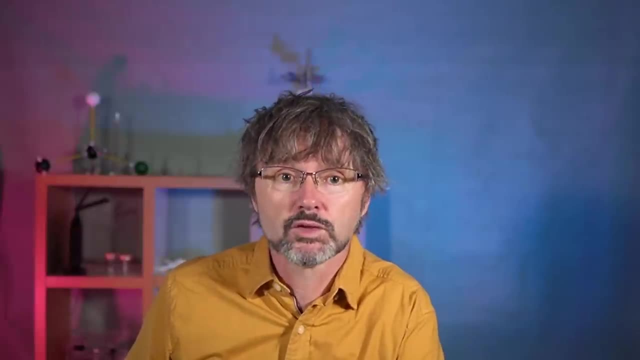 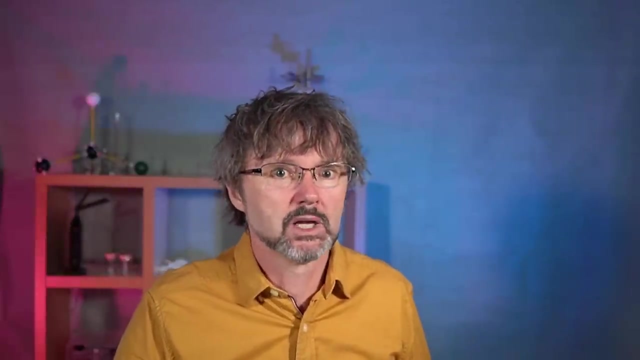 While related non-aromatic molecules are, for example, also populating the anti-bonding orbitals. The symmetry of benzene makes it a great molecule for visualising how molecular orbitals work. As before, this is not literally what's happening. 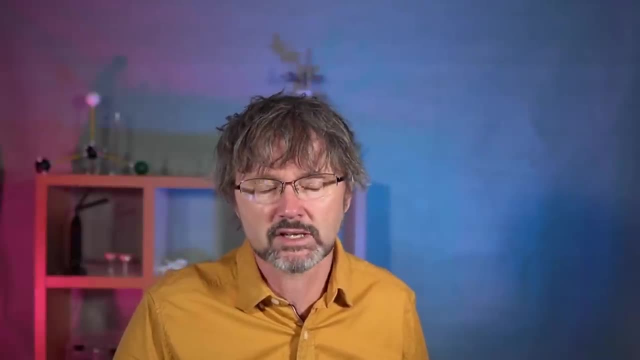 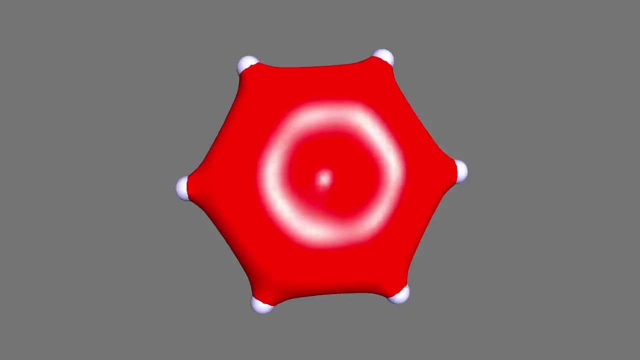 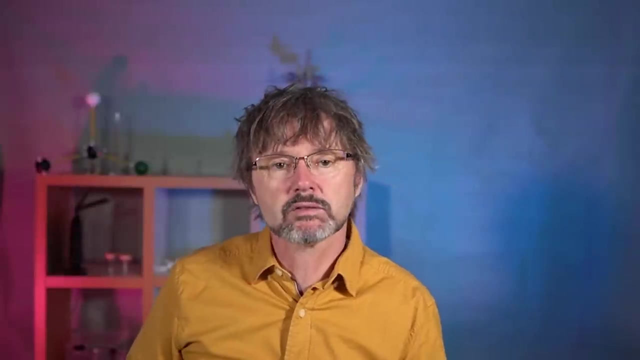 but it helps us understand the importance of symmetry and what the phases mean. If we look at this bonding orbital, we can represent it as one big red balloon or lobe stretching right across the molecule. Well, that balloon represents a single standing wave doing something like this. 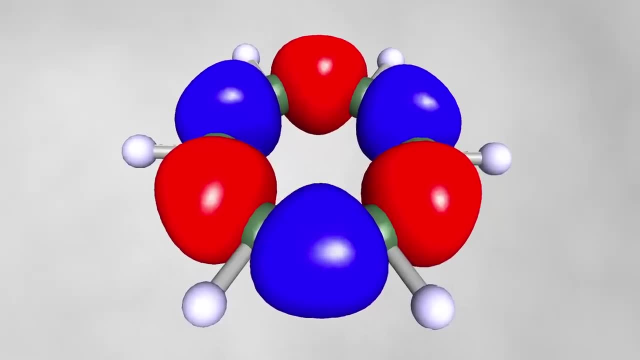 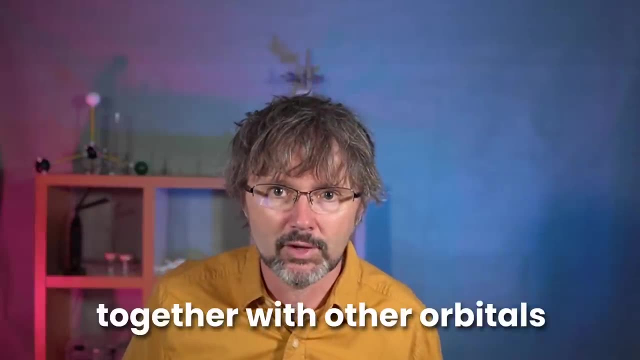 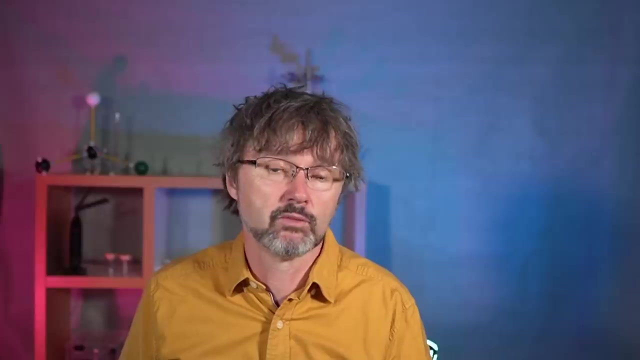 If we look at this bonding orbital, however, we get balloons between all the carbon atoms. In other words, it's holding the carbon skeleton together, But the lobes all have alternating red and blue colours. Those colours are saying that three of the lobes have one phase. 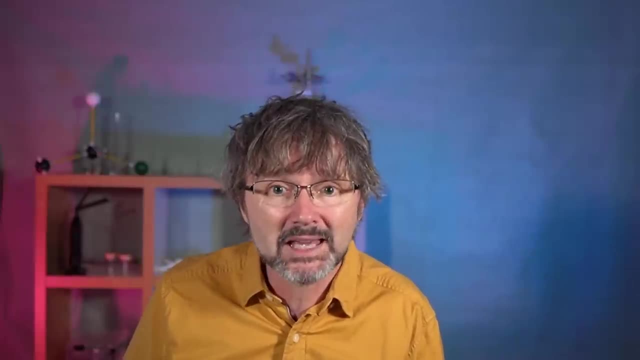 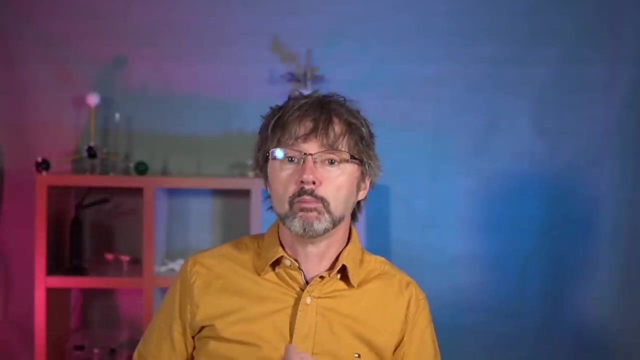 and the other three have the opposite phase. What does that mean? Well, it's something like this: Knowing about this theory, this symmetry right at the start, means that we can combine it with the rule of atomic orbitals, making the same number of molecular orbitals. 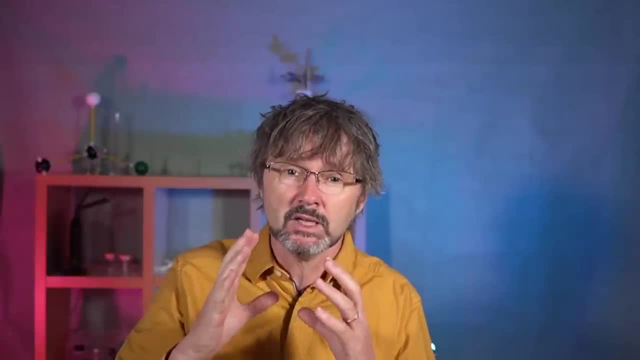 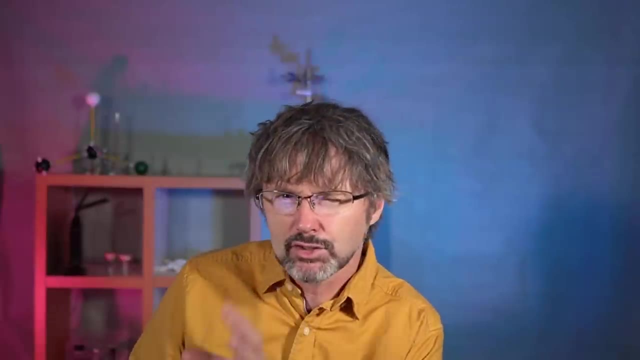 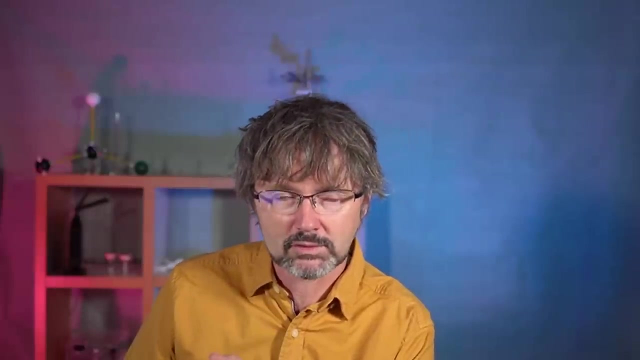 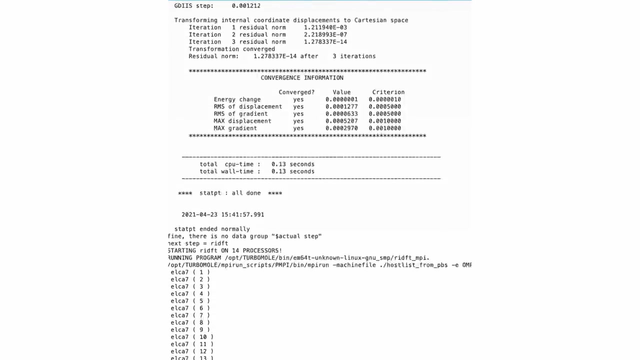 to really narrow down the possibilities when we're trying to calculate what molecular orbitals could be made. Now I should say here that theoretical chemists don't actually care about the shapes of these orbitals. They're only interested in numbers, Like what the energy differences are or the number of unpaired electrons. 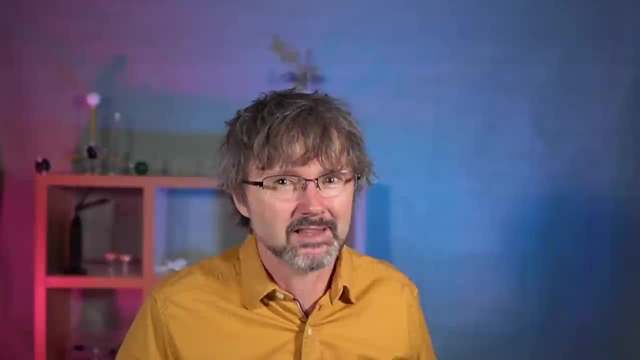 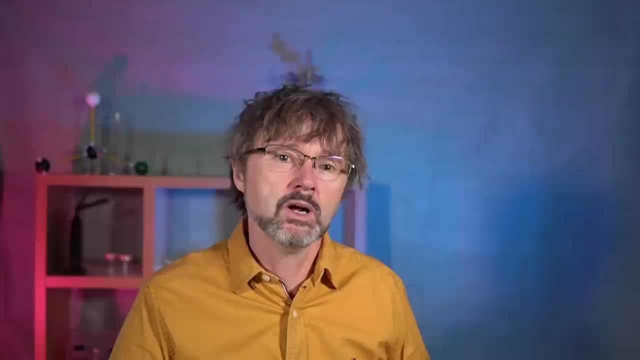 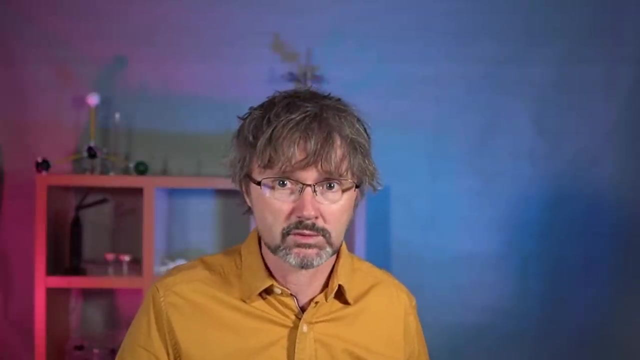 Which is a shame because they miss out on treats like this non-bonding orbital for benzene- What a beauty. Chemists designing molecules, however, are more interested, But even then they're mostly interested in the combined effect of all the orbitals. 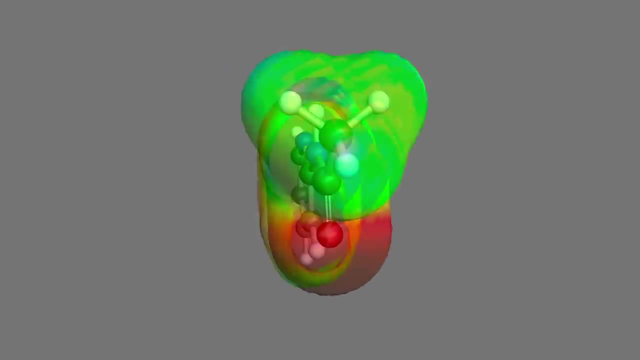 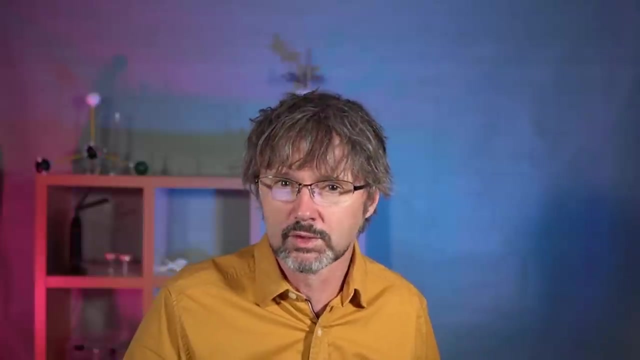 In other words, where are the areas of high or low electron density? Where are, or aren't, electrical charges going to show up on a molecule? The one time designers do care about the shapes of orbitals are for what we call the frontier orbitals. 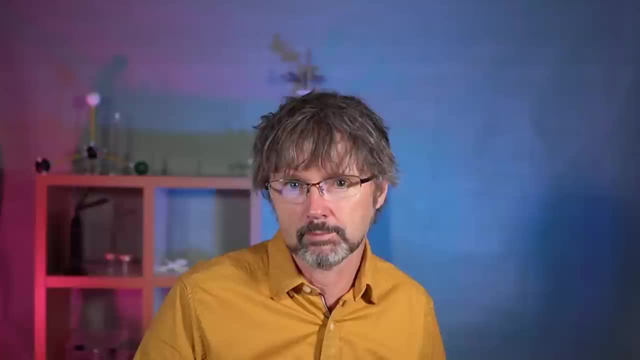 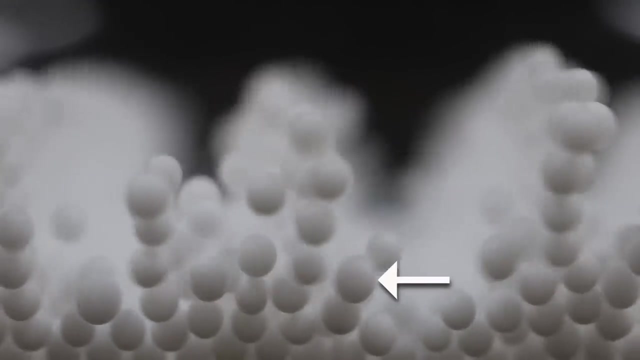 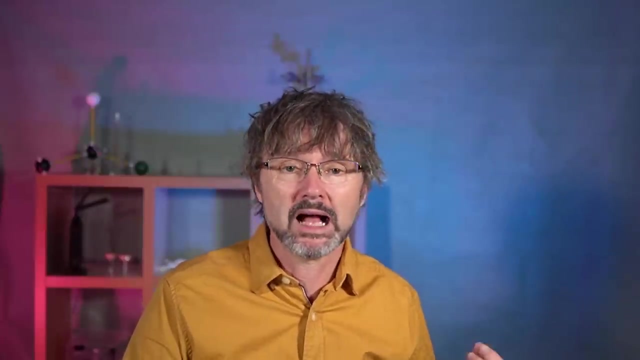 which is where most of the chemistry is going to happen. Electrons with the highest potential energy are the least stable ones. Things fall off the top of a pile right, So one of the places that chemistry will happen on a molecule is the molecular orbital that has. 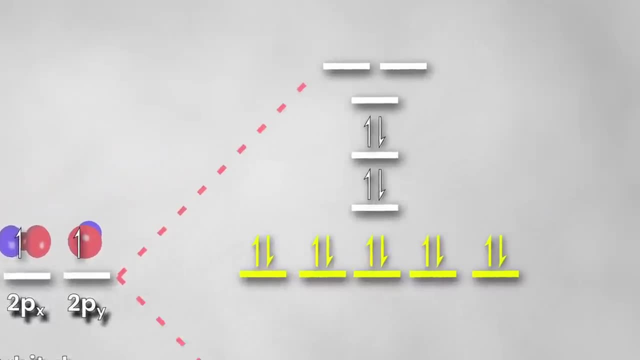 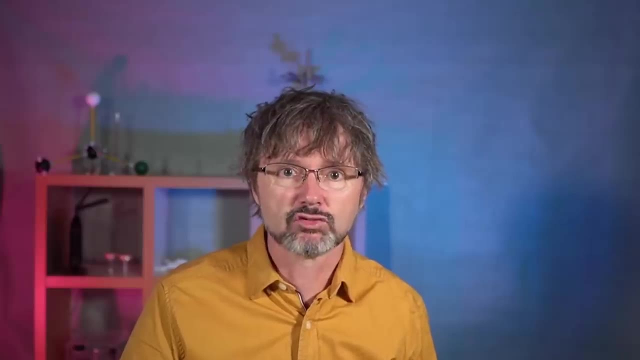 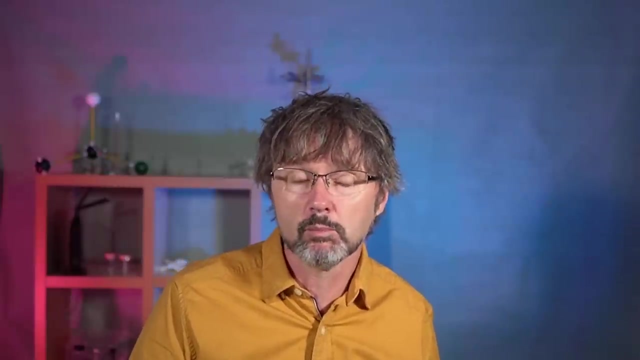 electrons with the highest potential energy, And this orbital is called the highest occupied molecular orbital, or HOMO for short. Now, electrons usually move into empty orbitals, So we're also interested in the empty orbitals of a molecule with the lowest potential energy. 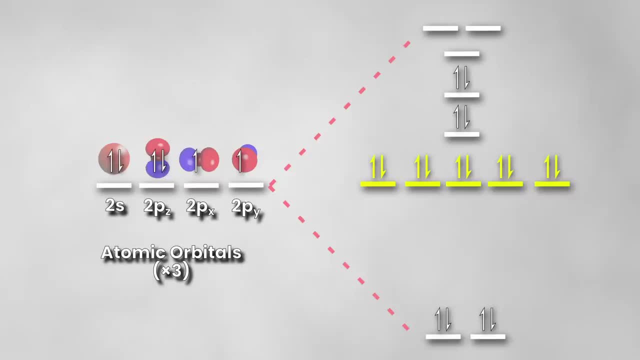 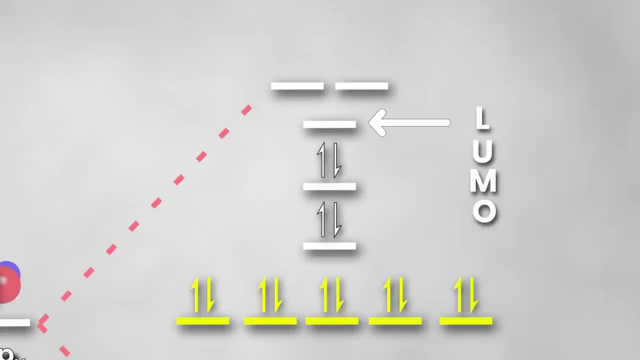 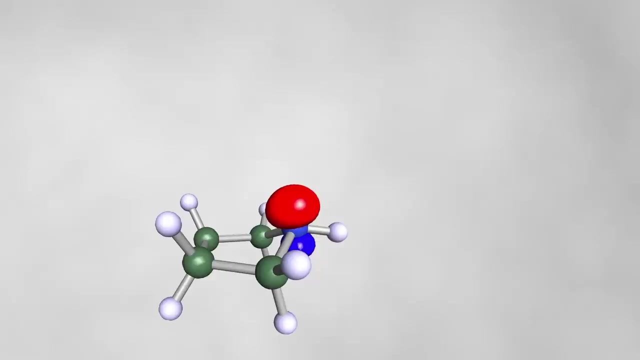 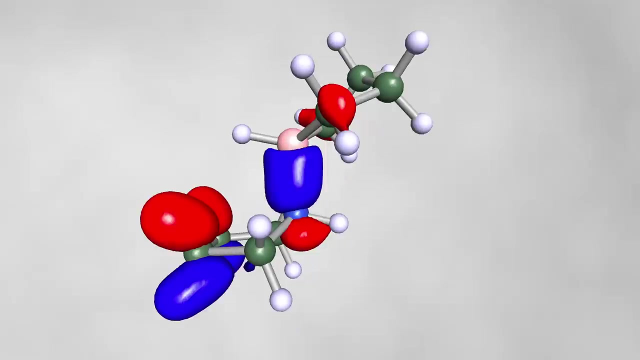 Because that's the easiest one for electrons to get into, And this orbital is called the lowest unoccupied molecular orbital, or LUMO. So, for example, in a Lewis acid-base reaction, electrons from the HOMO orbital of one molecule will be injected into the LUMO orbital of another molecule to make a new chemical bond. 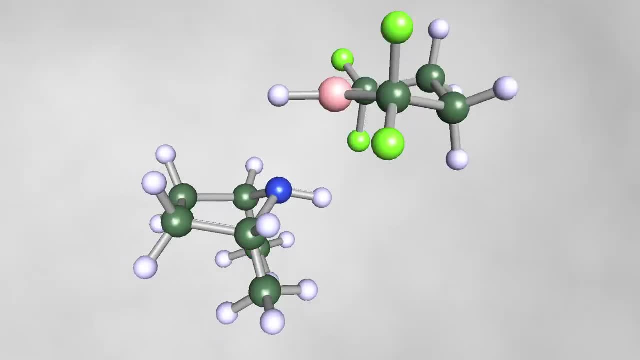 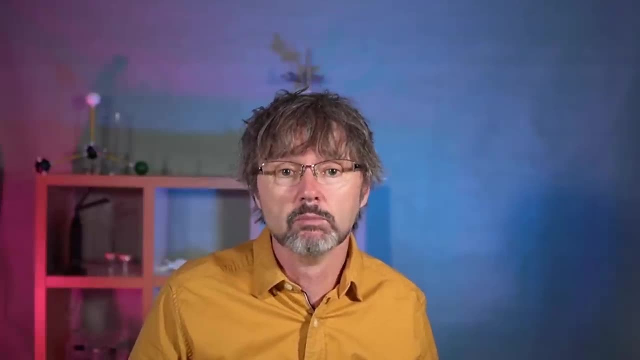 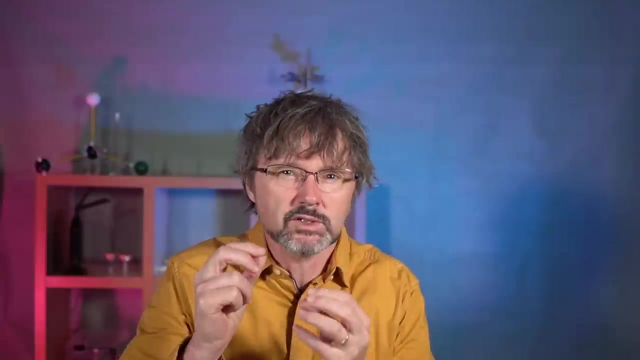 Chemists will change the atoms around these HOMO and LUMO orbitals to make their reactions faster and more efficient, or to make the products more stable. When we design catalysts, on the other hand, we'll be making fine adjustments for a kind of dance. 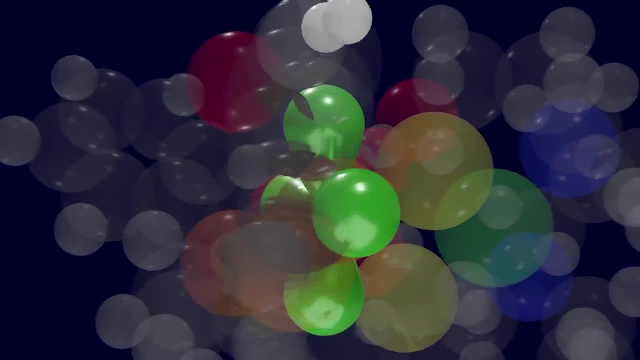 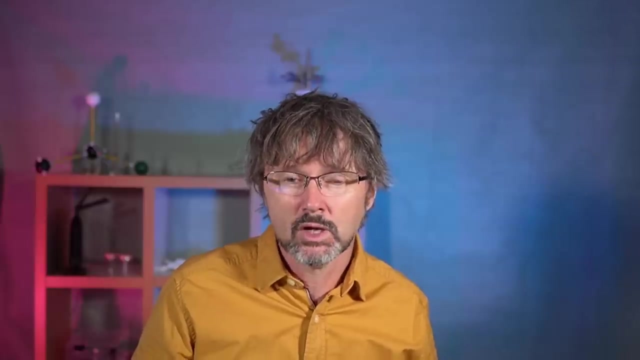 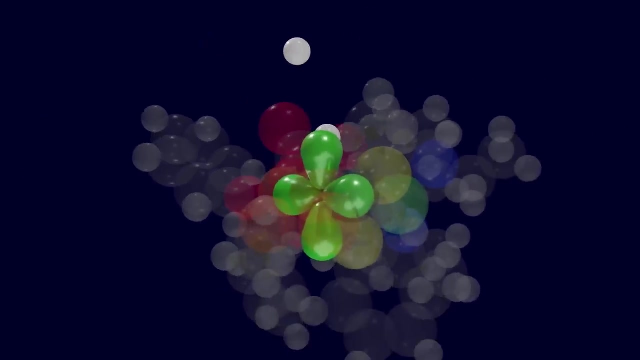 The catalyst might need a low energy LUMO to entice the reactants in and disrupt their stable molecular orbitals, while at the same time keeping a high energy HOMO to make sure the complex is unstable enough for the products of the reaction to get free. 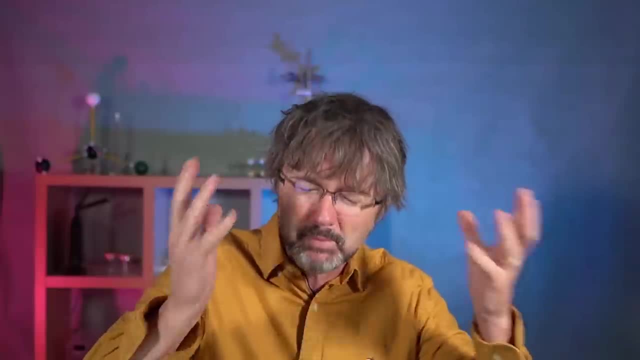 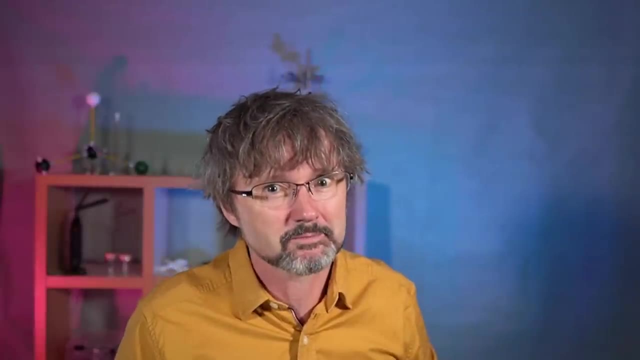 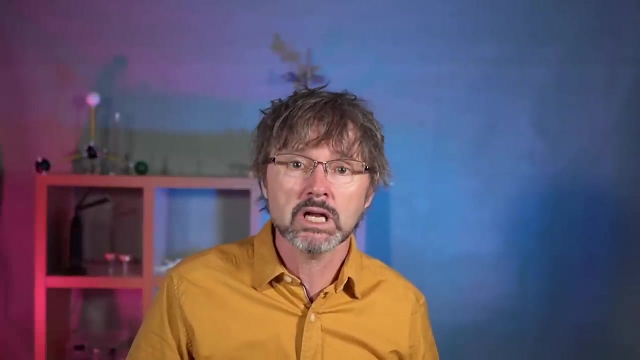 And getting that balance right is every bit as difficult as it sounds. Want a video about designing catalysts? Let me know in the comments. Another important point is that the difference in energy between the HOMO and the LUMO in the same molecule represents the smallest amount of energy. 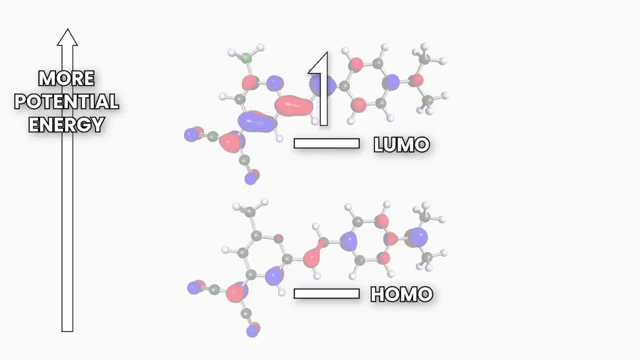 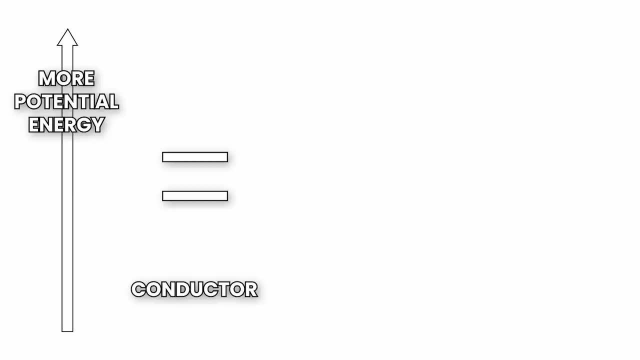 to excite an electron from one orbital to another within a molecule. In electrically conducting molecules we want that energy to be as low as possible, so electrons can flow easily from occupied orbitals to empty ones, And in insulators we need the opposite situation. 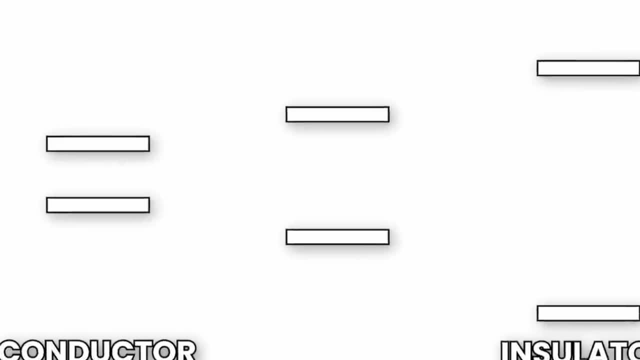 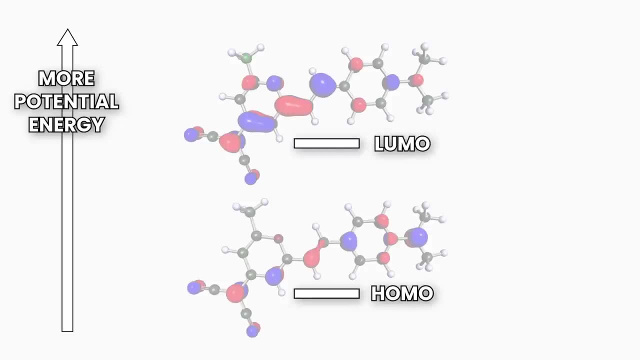 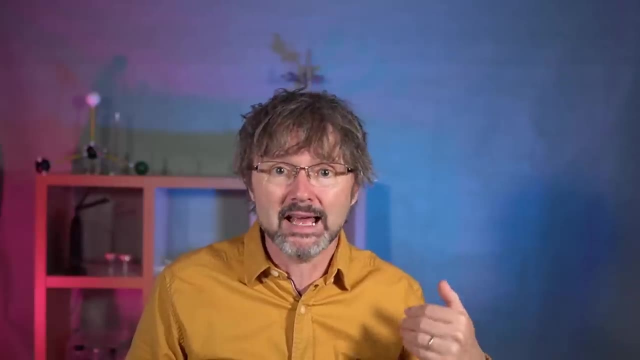 But it's the in-between cases where the fun stuff happens. Organic LEDs use this HOMO-LUMO gap by using an electric field to excite an electron from the HOMO to the LUMO of a molecule. The electron drops back down again almost immediately and when it does, it loses that. 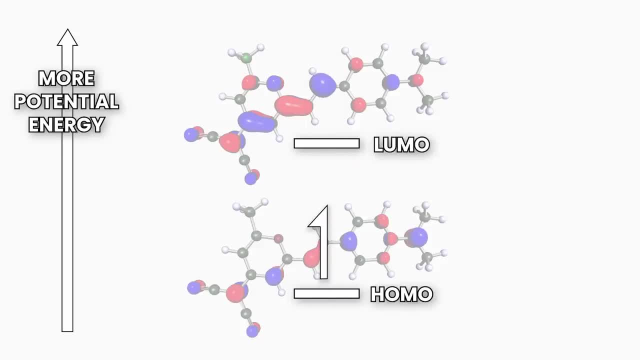 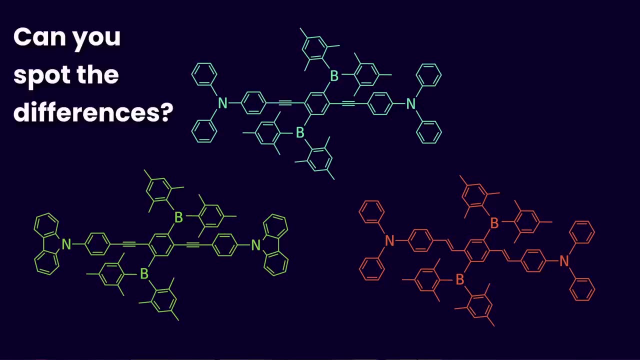 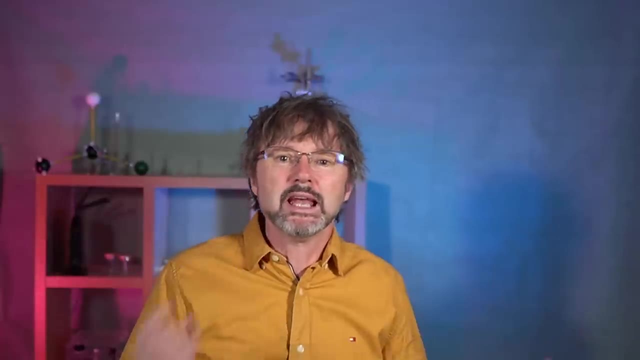 extra energy as a photon of visible light. So chemists have to design those molecules very carefully to finely tune that energy gap and get just the wavelength we want for a particular phone display, for example. Alright then. so molecular orbital theory is cool and better than valence bond theory. 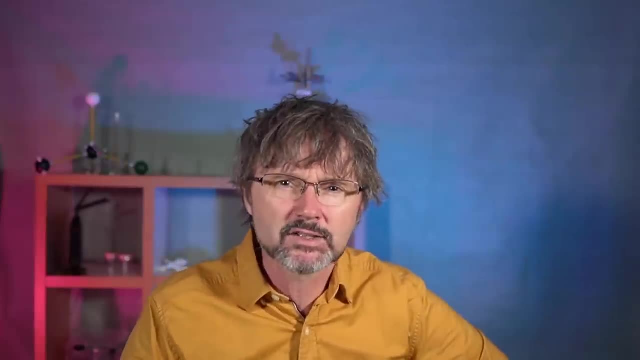 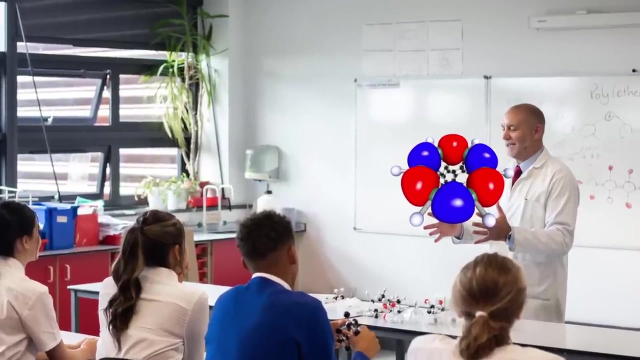 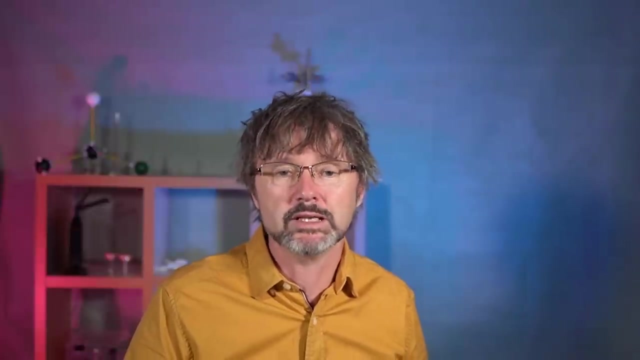 and Lewis diagrams. But if it really is so wonderful and better and fancy-pantsy, why don't we just start there at school? Why do we still learn all the other stuff? Well, very simply, as so often in science, we have to make a choice between usefulness and accuracy. 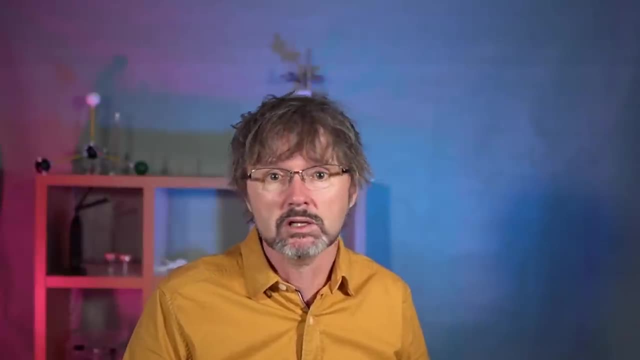 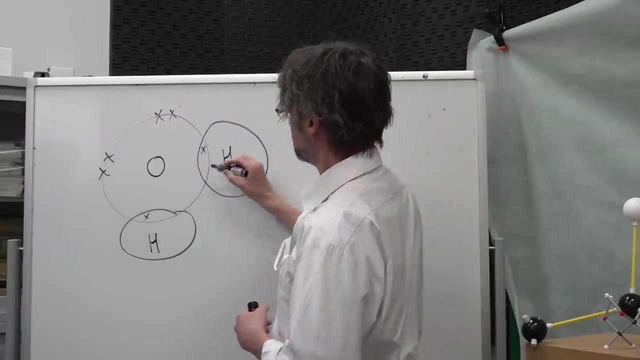 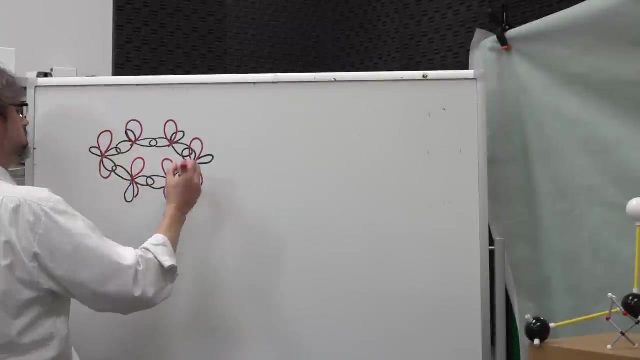 For most people who only study chemistry at school, Lewis diagrams are fine for understanding the basic rules behind how atoms make molecules, But at university we need a deeper understanding, and so we move deeper into valence bond theory with hybrid orbitals. It's more complex, but you can still do it in your head. 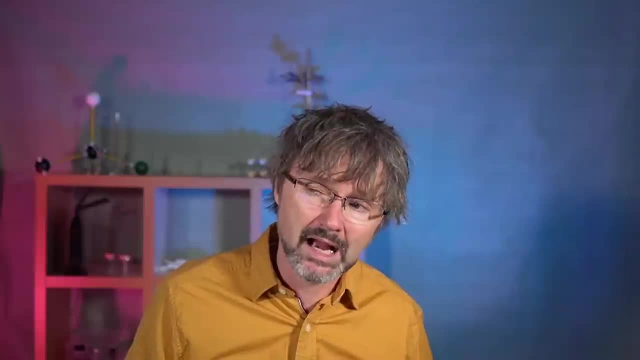 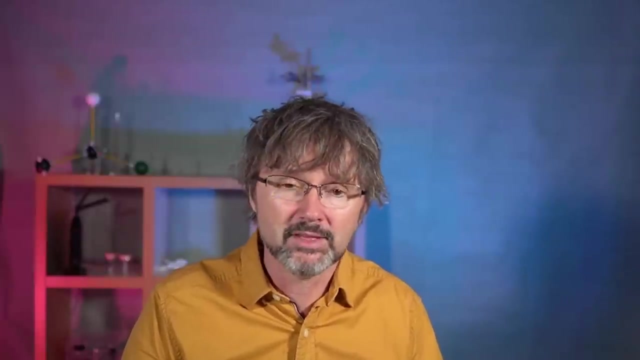 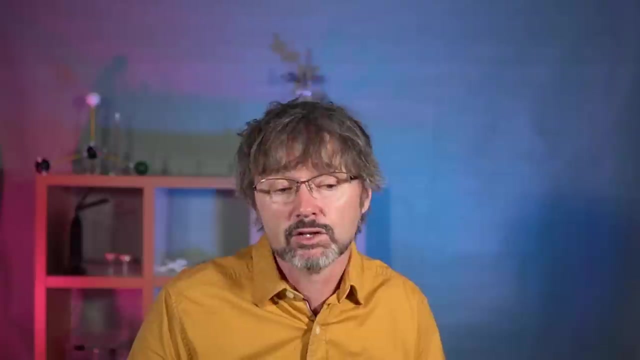 And yes, molecular orbital theory is much more accurate. It makes better predictions and explains more phenomena than valence bond theory. But for anything more complicated than small molecules you need a computer to calculate the properties properly. Using valence bond theory I could have talked about all of these molecules using only a whiteboard. 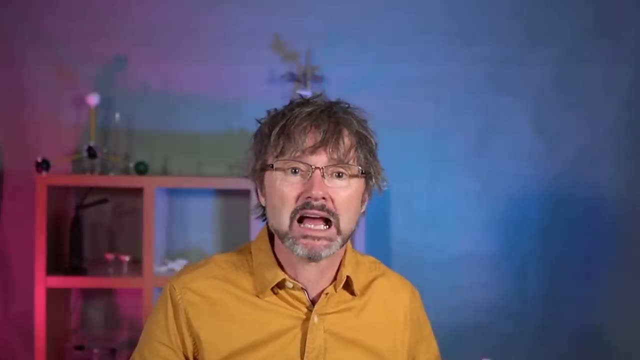 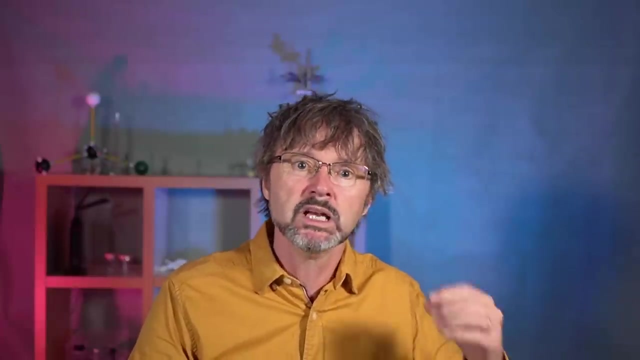 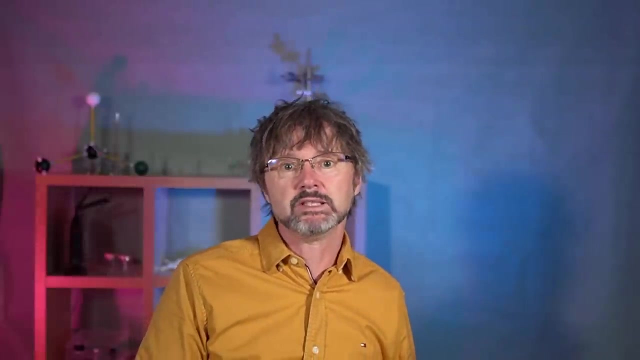 But, most importantly, valence bond theory is a VSM, So I can do a lot of work without having to use a calculator. bomb theory allows us to use our qualitative brain, our visual imagination, and that's important, because so much of chemistry is an imaginary visual science, So theoretical chemists typically 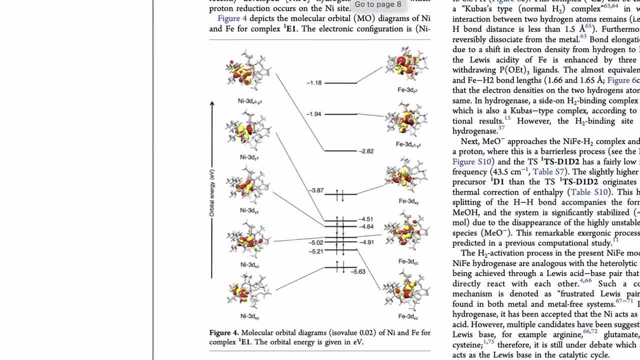 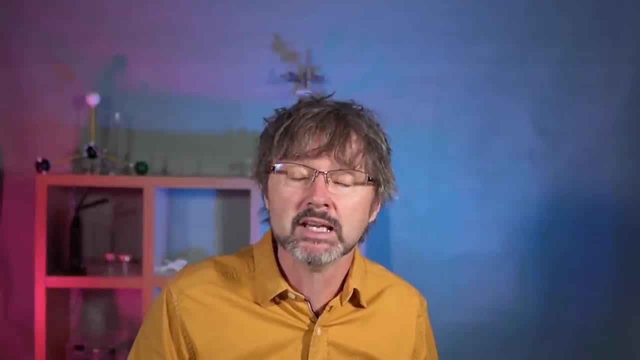 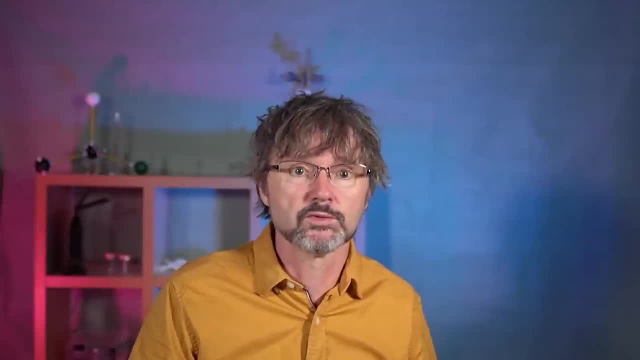 work in tandem with synthetic chemists to get the best synergy of the two ways of thinking. So the different approaches to molecular theory each have their own advantages and disadvantages, And so, in practice, we use the best tool for the job. That said, 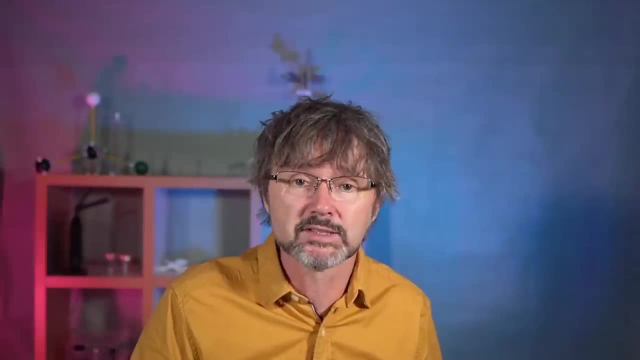 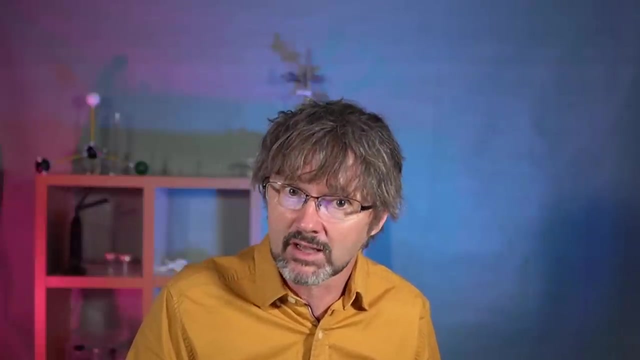 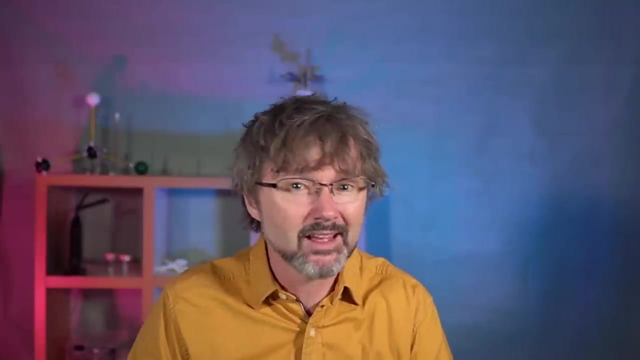 valence bomb theory is making a comeback in the theoretical world too. There are some things it explains better than molecular orbital theory, but that discussion is for another day Now, at the beginning of the video I promised a resource for an academic course on molecular 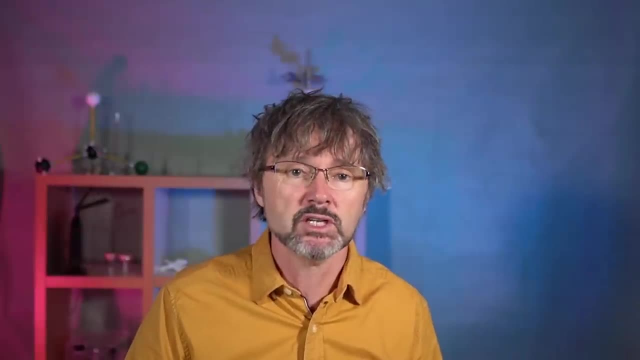 orbital theory. So I've put a link in the description to a great course on molecular orbital theory. So I've put a link in the description to a great course on molecular orbital theory. So I've put a link in the description to a great YouTube channel called Chad's Prep. His lessons are great, So check it out if you want to. 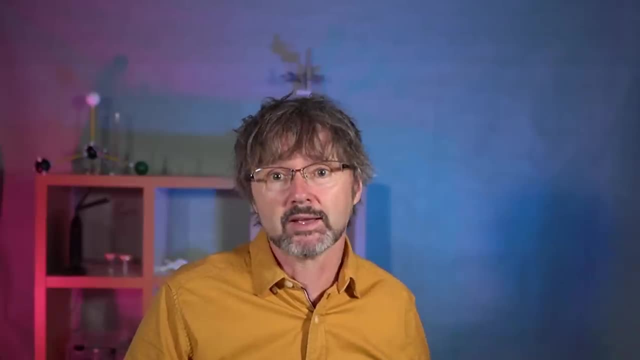 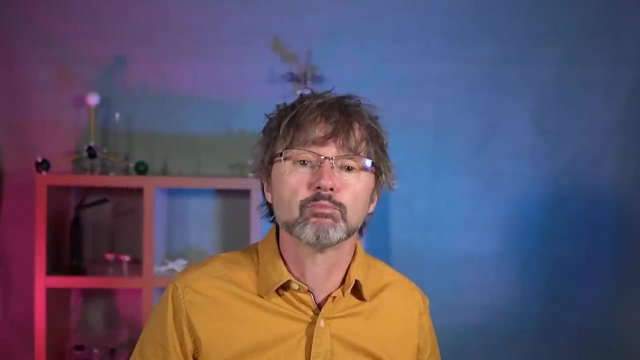 dig deeper. And why not tell him I sent you. So what do you think? Have you heard of molecular orbital theory before? Were you ever confused about it? Would you like to see how it's used in practice? Let me know in the comments. But why not hang around for the bonus extras? 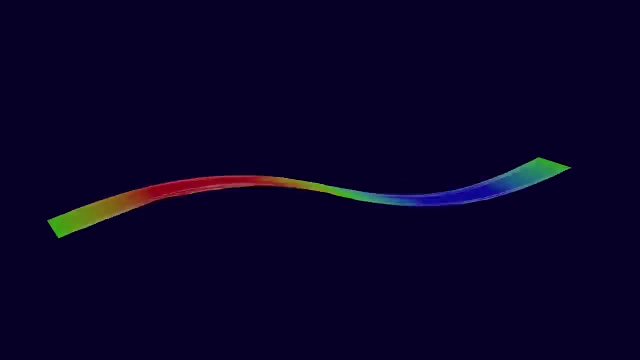 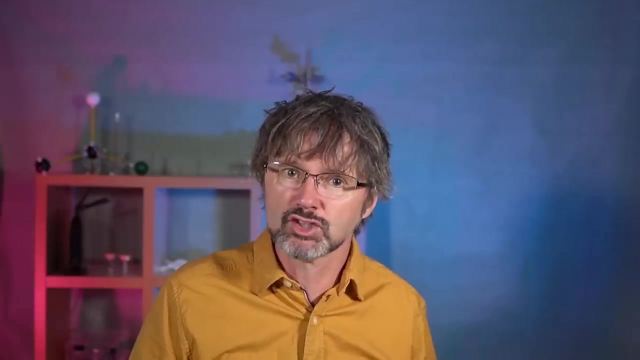 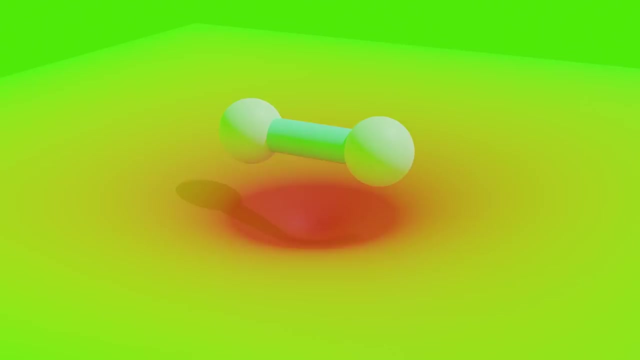 I showed you the vibrating ribbon as an illustration of how phases work in hydrogen. but there's a more accurate image if we use a two-dimensional sheet and imagine that it extends to the end of the universe. Now we can see that the oscillation doesn't magically stop. 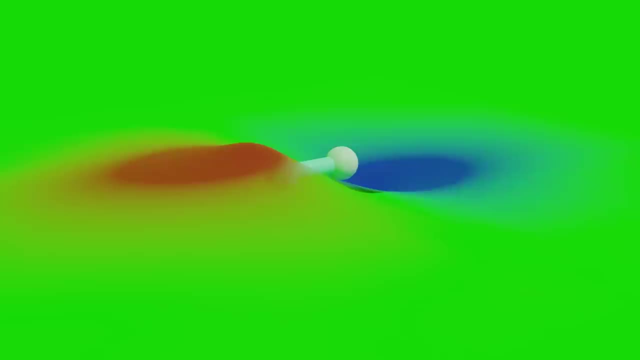 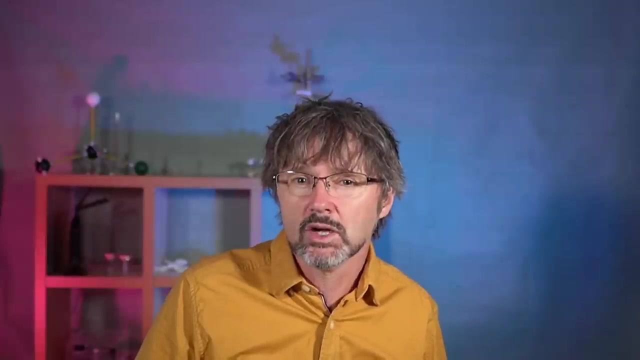 at the end of the molecule but extends outwards in all directions, basically forever. But there's a point relatively close to the nucleus where that oscillation is no longer significant, And that's what we call a single molecule. And that's what we call a single molecule, And that's what we. 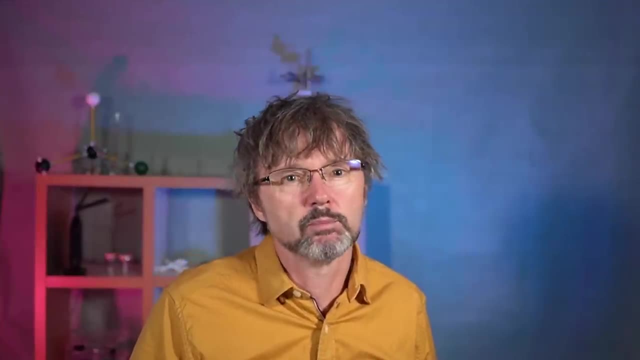 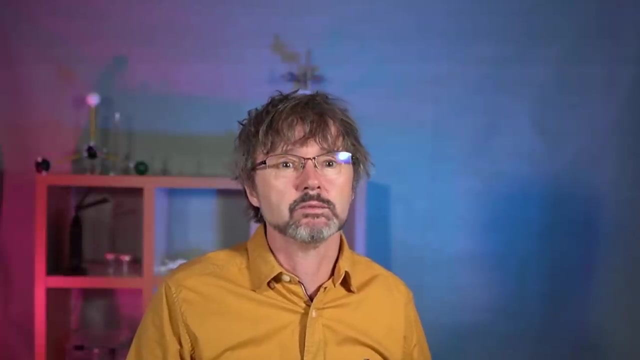 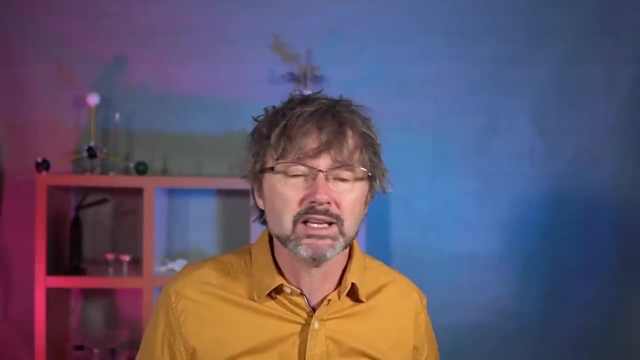 call a single molecule. The next, and probably most important point is that when we get down to the size of atoms, and especially electrons, it simply isn't possible to imagine them clearly. We can call them particles or call them waves, but they're not truly like either of those things, So we need to 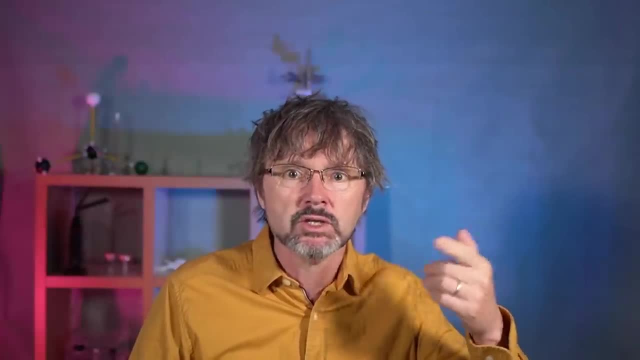 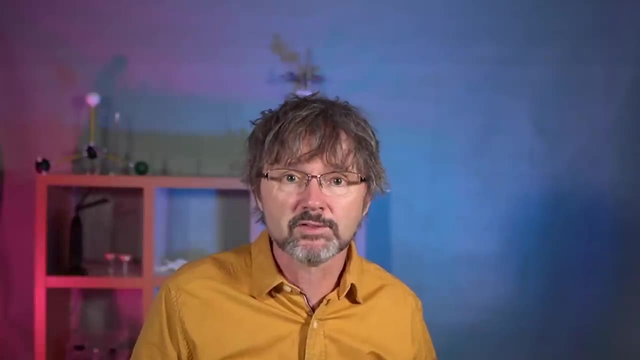 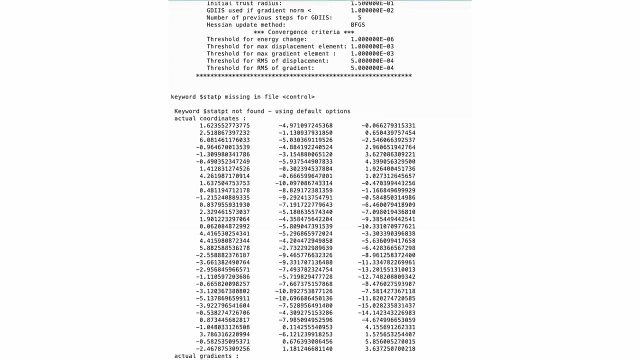 make models using our qualitative imagination or mathematics, and those models will always be flawed in some respect. So what we have to do is to choose a model that works best for our purpose. Some are simpler, some are more accurate, but none of them is universally better. In chemistry, we usually 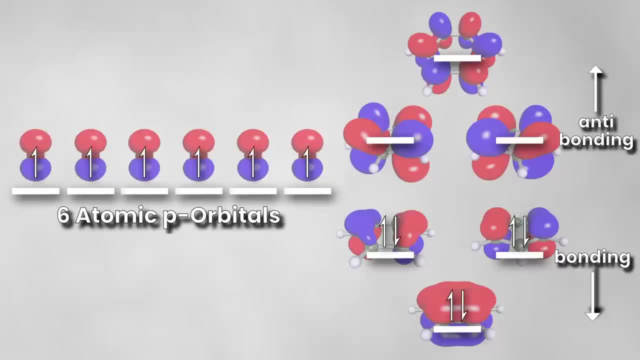 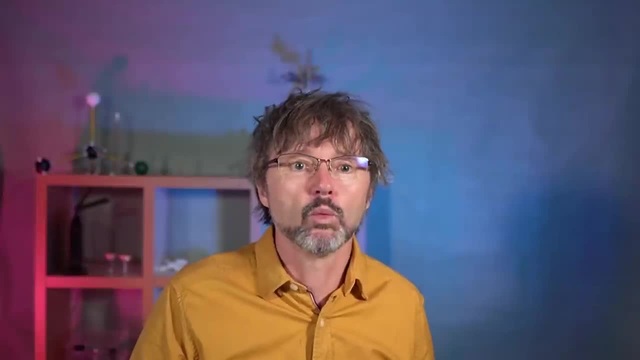 talk about electrons and orbitals as being separate things, but that's not really true. In quantum mechanics, the orbital represents the combination of the wave nature of an electron and its particle nature. And no, no one can really tell the difference between the two. 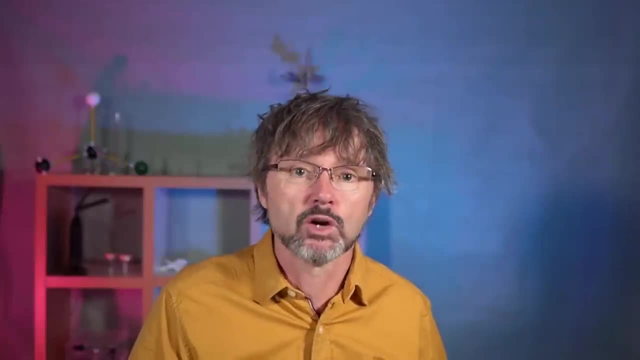 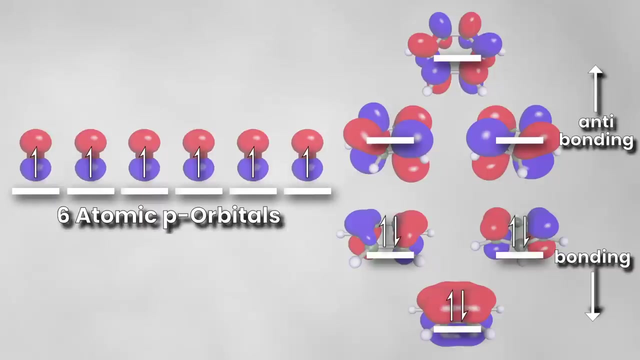 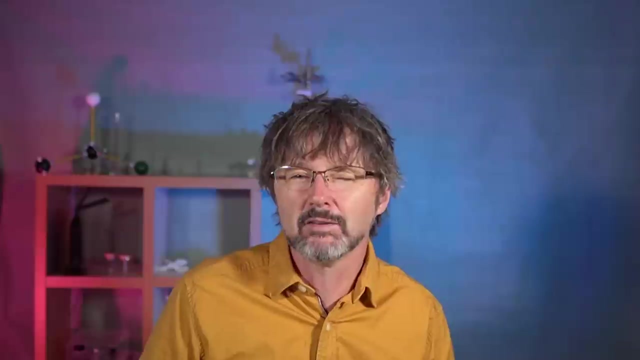 So electrons as particles sitting in oscillating spaces called orbitals is simply the most useful model for chemistry. But if you have a good way of explaining molecular orbitals, I'd love to see it in the comments. See you next time.